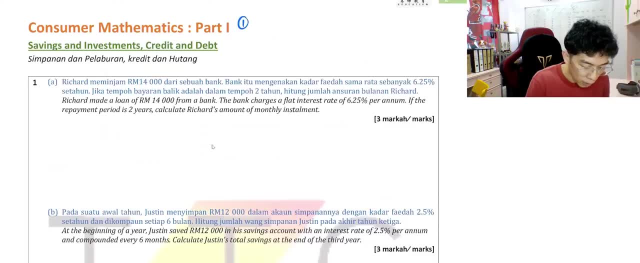 it Now the first thing is. the first thing is I want you to write the word interest. Okay, write the word interest. And once you write the word interest, right, I'm going to straight go into the information that I compiled already and make it into your form. five kind of revision: 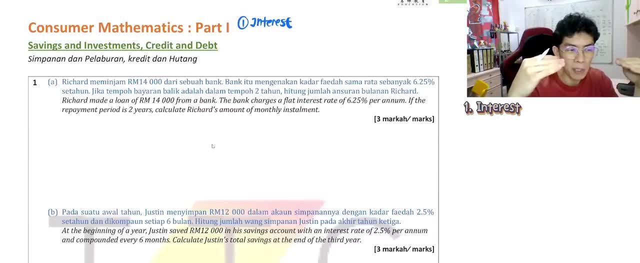 Because during form three you will say something like teacher. I remember interest got like a few types you know, like simple compound, then loan got interest, some more, but two different categories. Why? Because your simple interest and compound interest is about receiving the interest. 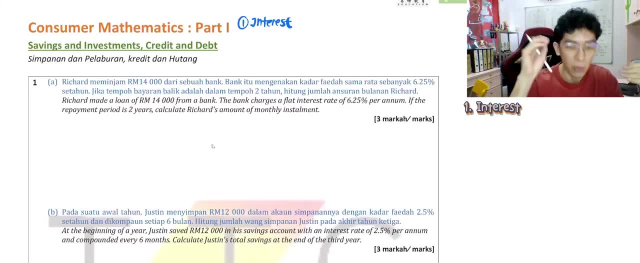 And then, as for the loan related interest, it's about you paying the interest to the bank, But anyhow, the calculation is the same. Okay, so we're going to go into, like the interest related stuff, And the first thing being the simple interest related formula. So can you put simple interest? you can. 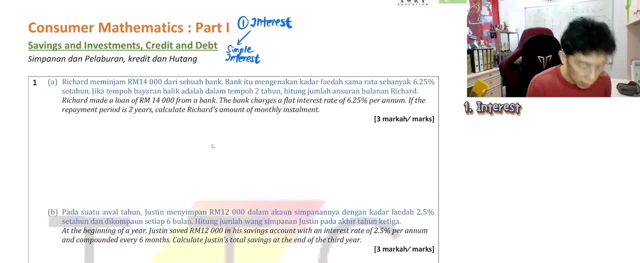 start writing it already. Okay, so simple interest, the formula. what is it about the formula? I'm not sure whether you remember or not. I'm pretty sure you remember it. Come try. What's your simple interest formula? Okay, so interest equals to PRT. What is P Principle? or maybe deposit, R being the rates, T being 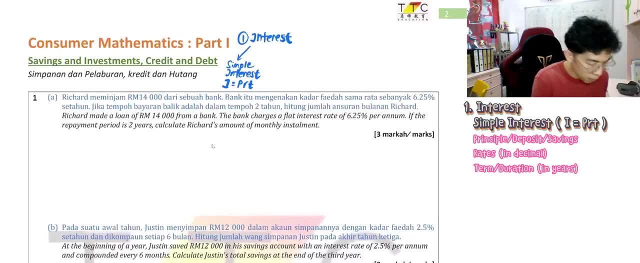 the term Term means how many years? Okay, just a quick one, everyone Remember: 20% indicate 0.2.. How about 2%? Tell me in decimal point, what's that? Yes, fantastic 0.02.. How about 100%? everyone? 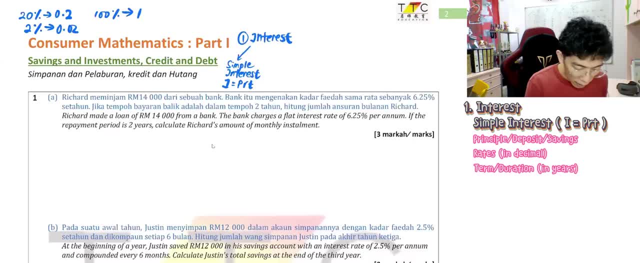 Simple, right One. So you know all these things Okay. then we have another one called compound interest. Okay, compound interest, this thing. So later I will go in depth on what is compound interest. In case you forget, really later you can ask me, teacher, what the hell is that? 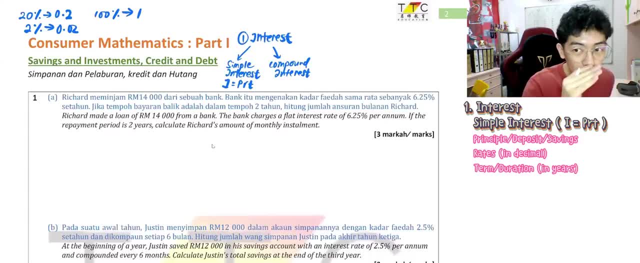 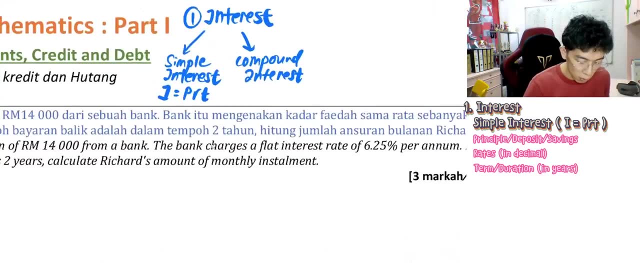 But I will give you the formula first. And what's the formula for compound interest? By the way, there will be formula in your SPM: It's given really. Okay, it's given really. So now let's go. Let's go. Your compound interest related formula: it starts with N. 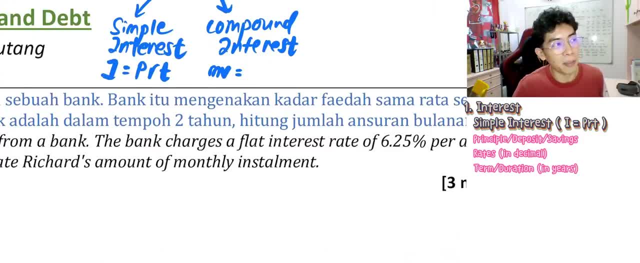 V. Come tell me what is N? V. But don't worry, because once you know how to do right, you don't even need a formula right. So I will go through it. Okay, so you all manage to like. 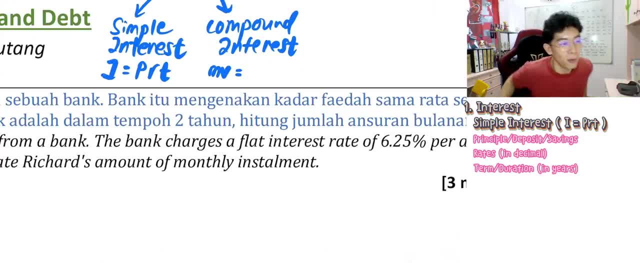 remember it. Nice, Then you don't need the formula anymore. Yes, what is N V Come, Thank you. N V stands for matured value, Matured value meaning what It means. let's say a particular example: FD, fixed deposit. So you're going to place your principal of 10,000,, for example, 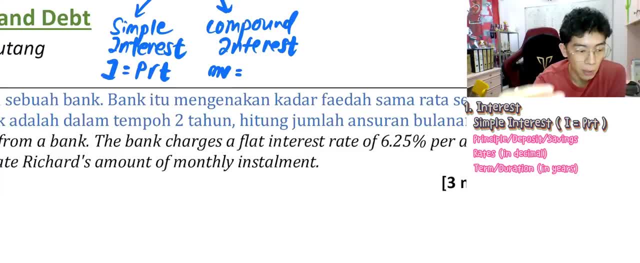 and you place it inside and you plan to save it. Okay, plan to save it for three years. So after three years, the total amount including interest compounded inside, that's your matured value. That's the one, Okay. so what's the formula for this thing? I like watching pro Heaven say: 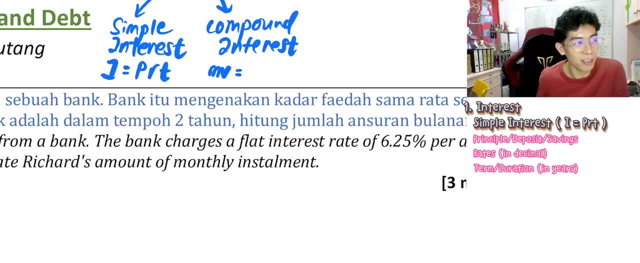 really give answer Next level already. Xuebao, Okay, come, So come. Aina, come, Okay now. so the answer is P, open bracket. Okay, P stands for principal, of course. Now I'm going to say the one. The formula is about P, bracket one. What is one? 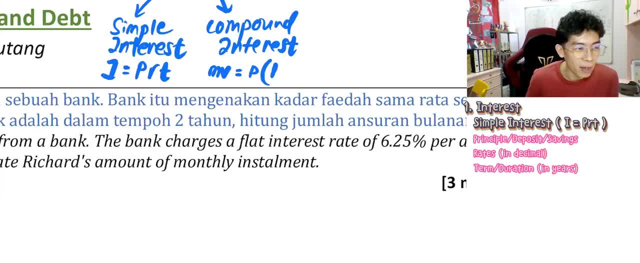 What is one? One means 100%, And the 100% is actually representing the principal principal amount, Re representing the principal amount. then you add up with R divide by N bracket NT, then students scratch their head. Teacher cannot, la. what kind of thing is this? 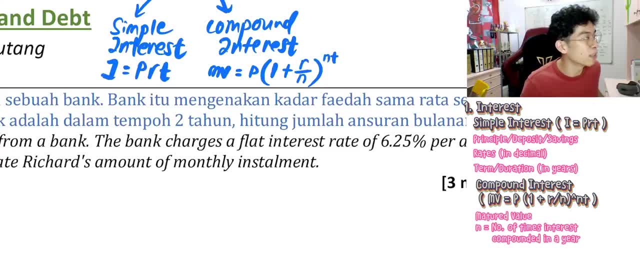 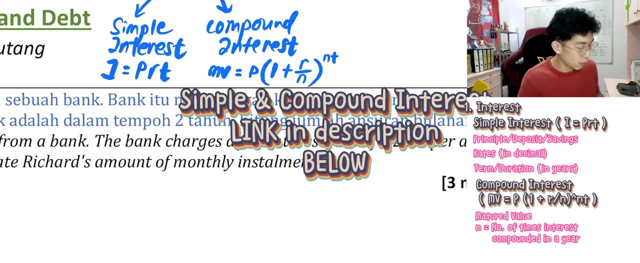 Okay, I'll show you. okay, I will show you And simultaneously I will send you, like the video that I made it before. Okay, so I sent to everybody. ding, Okay, sent for fun, only one, Okay, so come back. come back Now, then. this is about the two. 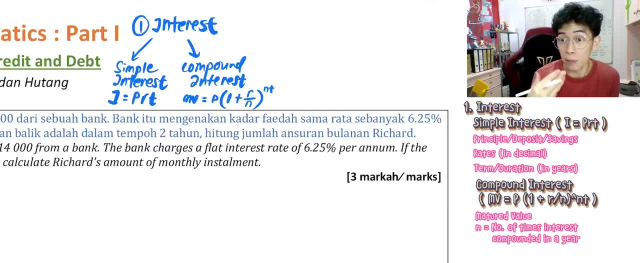 interest where it's about receiving it- you receiving the interest- and next we have another one where it's about loan related interest and loan related interest, or basically it's about simple interest. you know you're going to use the PRT thing, but I'm going to change a bit. 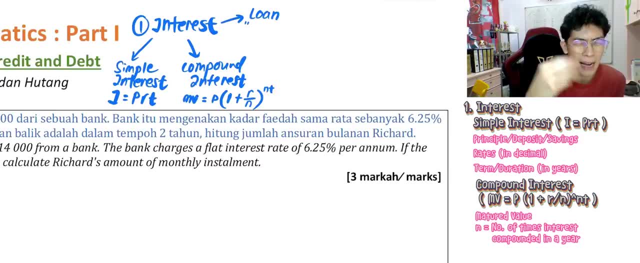 and under this loan category, most of the time they are asking about: hey, can you find me? the total repayment of the loan. the total repayment of the loan including interest. so what is that formula? I show you. I show you. you see, whether you understand or not, P plus PRT, everyone let 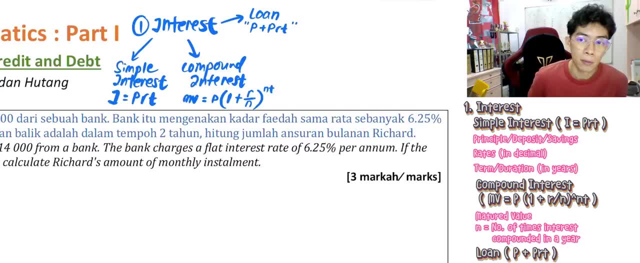 me ask you all. you all tell me what is P. I know P is the principle, right, but in loan point of view it means what P is the principle? yes, so in loan point of view, what is the P? P stands for the amount that you're going to pensando from the bank. you go bank there. 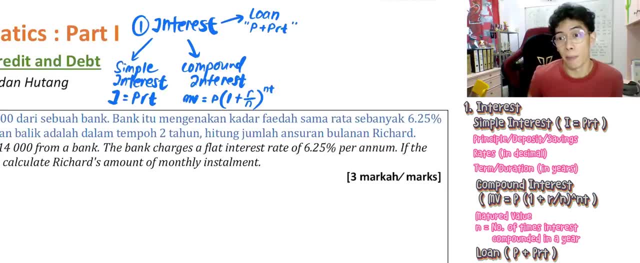 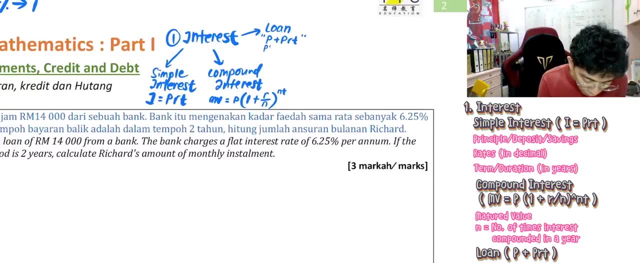 hey, bank, I want to pinjam 10,000.. That's the principal amount. Okay, can so the starting value, starting value, Then the PRT thing, it will be the interest. So this is the principal and this is the interest. 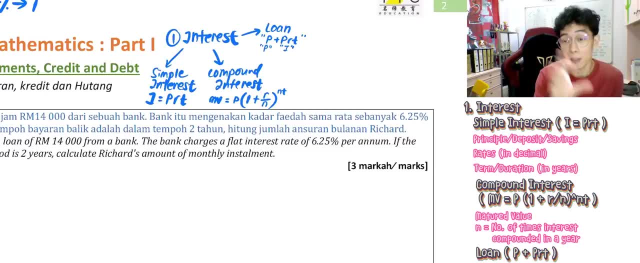 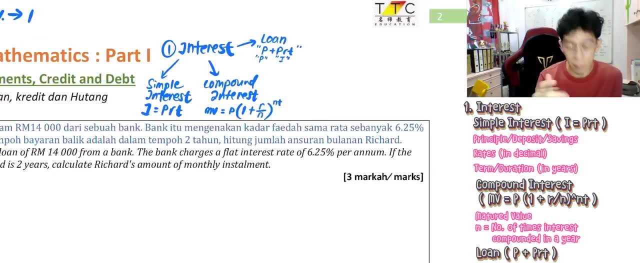 So this interest. you have these three very important part that you have to know. So later I will go through the questions about these three parts. Then the second part that you need to know under consumer mathematics, the second part, by the way, these are Form 3 related stuff. 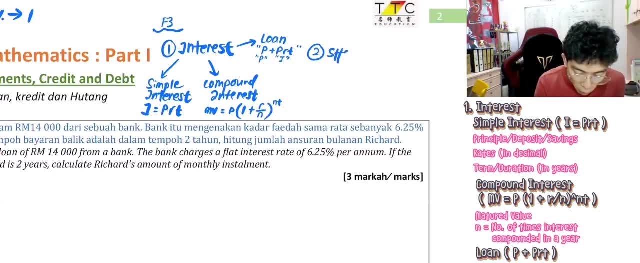 I'm writing it over here. Then the second thing is you have to know something called the shares. Okay, the shares. So everyone tell me another name for share. Another name for share. Okay, yes, I know, it's Saham. 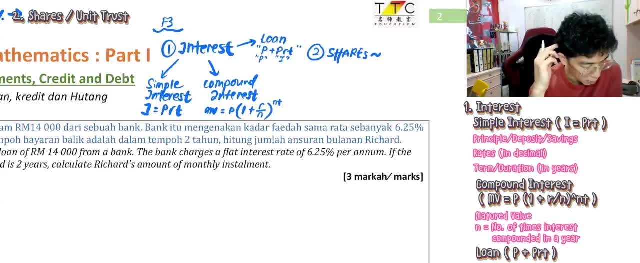 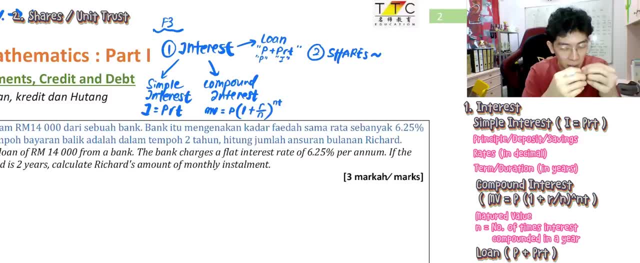 we don't really go super in-depth, We just categorize in two different categories. The two different categories will be just a normal shares that you're going to buy it yourself, And the second part is about unit trust, Everyone, supposedly these two things. 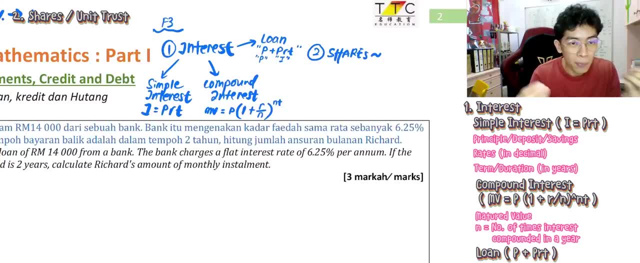 are two different stuff, But under our Form 3 category it's roughly the same thing. Question-wise also the same thing. If they say shares they see unit trust. same thing In Form 3 categories, It's just that what's the difference? 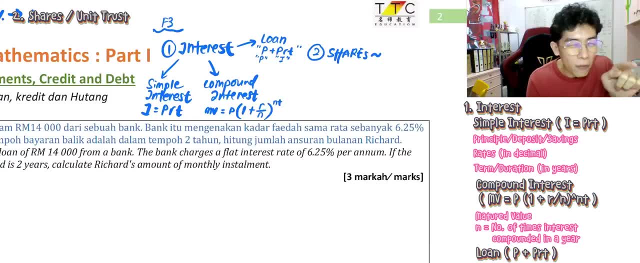 The difference will be: share- you buy it yourself. Unit trust. who buy it for you? Professional manage for you. Unit trust, you're right. Professional manage for you. You just tell the professional: hey, professional, I'm going to invest in shares. 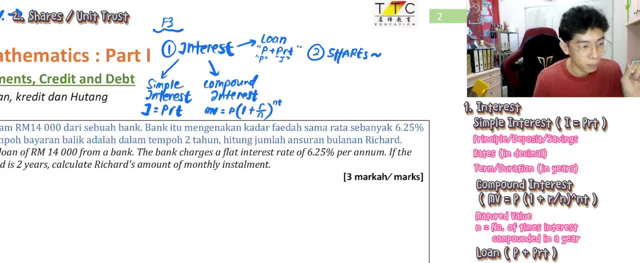 Can you settle for me? Okay, I settle for you, So that's the one. Then under shares, right? You will say something like: oh, I repeat, Uh, let's say they talk about shares unit trust under our syllabus, right? 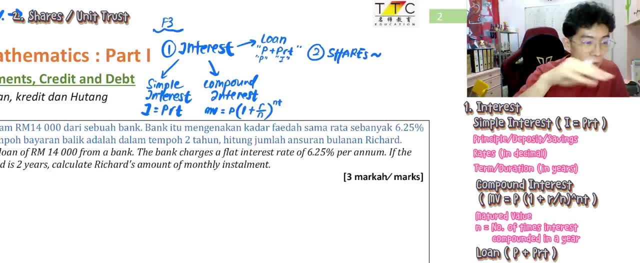 Calculation-wise everything is the same, It's just that we don't go really in depth. What's the definition of unit trust and like shares, all those things? No. So it's the same calculation And under this kind of share-related question, right? 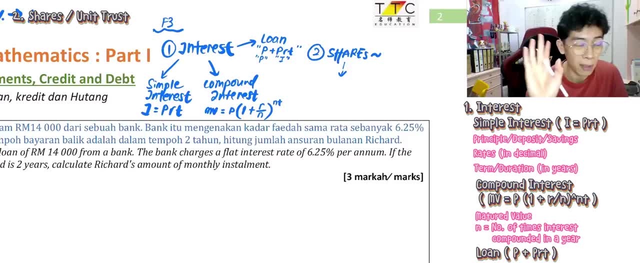 There is a few types are like dividends, how to calculate all those things, But that one kind of easier later when I do the questions with you. But the important one: it's about this thing called cost per unit And students kind of you know what. 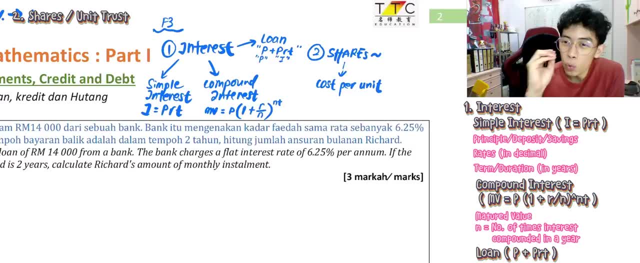 They just too, they get too worried, you know, and because you have to handle so many subjects, you know, and your tends to your tends to what you know, tends to focus too much on the exact word Teacher, why this question didn't write cost per unit one. 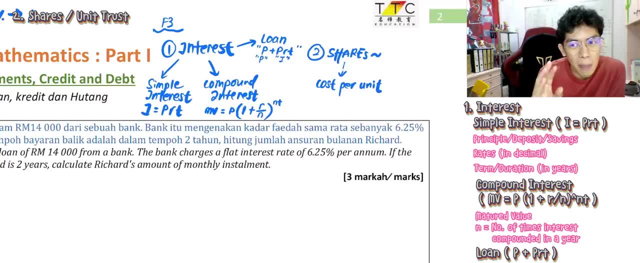 but instead of that write other names where it seems a bit similar, but I think it's not the same. So let me tell you cost per unit. you learn it in form one before, For example, for example. now listen up carefully everyone. 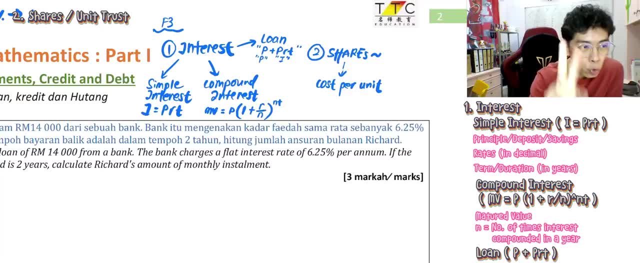 If, if I buy two G2 pens, I buy two G2 pens, the two G2 pens right Cost RM10 ringgit. What is the cost per unit for one G2 pen? Easy, right, RM5,. do you notice something simple? 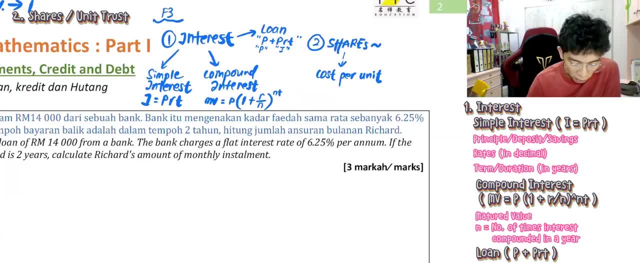 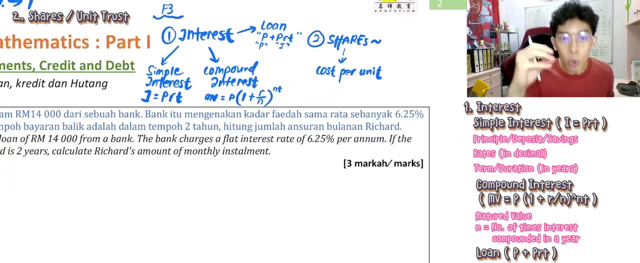 where even primary, you understand it before Then this cost per unit. if, let's say, I go real in depth, if I go real in depth, I'm going to tell you a story together with this very important thing. Come you circle this one. 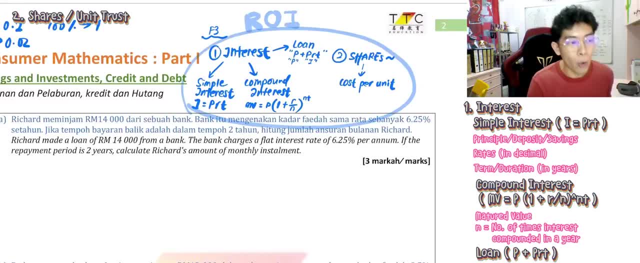 together with a very important thing called ROI. ROI can happen in both side. So this ROI, I'm going to ask everyone. see whether you get correct or not. What is ROI? I don't want to formule, right, I don't want to formule, I just want the name only. 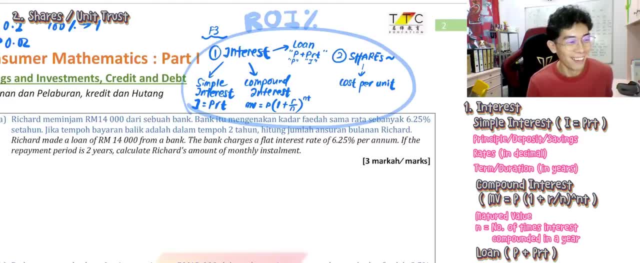 Formule. I'm pretty sure you forget already, la. Okay, The previous two class said the same thing. I tell you. Later I'll tell you what is that same wrong name that student told me. You see, you see now three versus three. 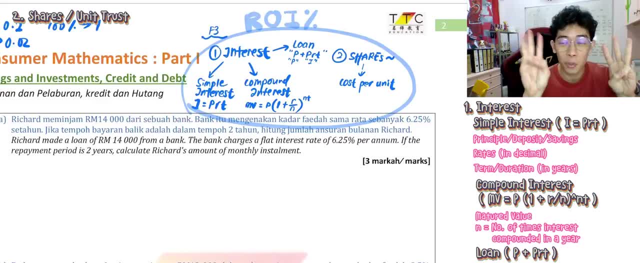 six student send me the answer already. Three student get this same answer and ah, four student get the same answer. now, Ah, Rainer, ah, you know you're wrong, right, Okay. then the other. ah, okay, five, five versus four. already you know. 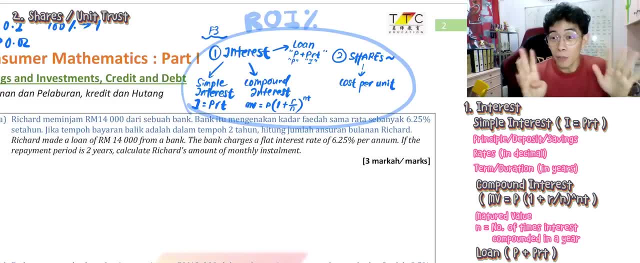 Come more. Okay, never mind, but never mind A lot of student, I don't know why. ah, ROI, they link to this answer, you know? Okay, now the wrong answer. right, it's rate of interest. 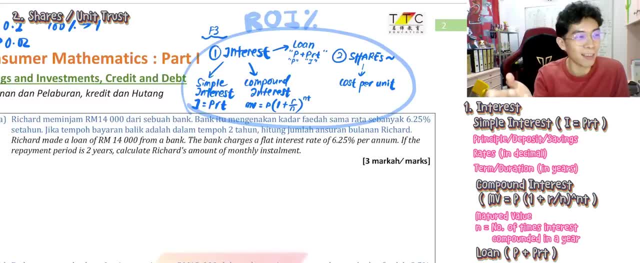 Cannot la. where got rate of interest one? People say interest rate one, ma where got rate of interest? Okay now. so ROI stands for what? Ah la ma. But it's okay la. you all forget already. it's normal. 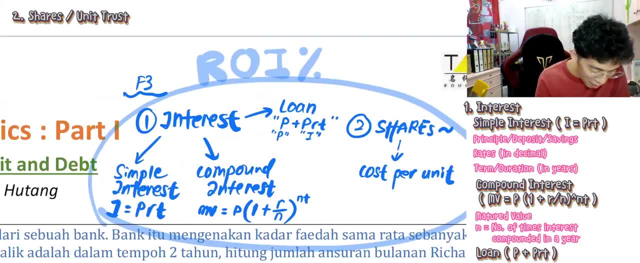 Okay. so the answer- yeah, Rainer, correct The answer- is return on your investment. Return on your investment, return of investment. Ah, so it depends on how you read it, la. return on, return off. same thing on. 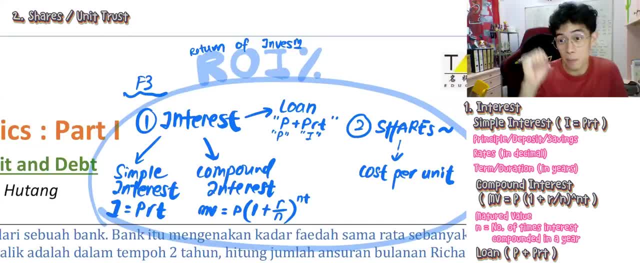 Ah, I repeat, ah, return on your investment, Return of your investment, your investment. okay, right, So I'm going to use one story to supple this cost per unit and ROI thing. Okay, now let me tell you: ah, see ya. 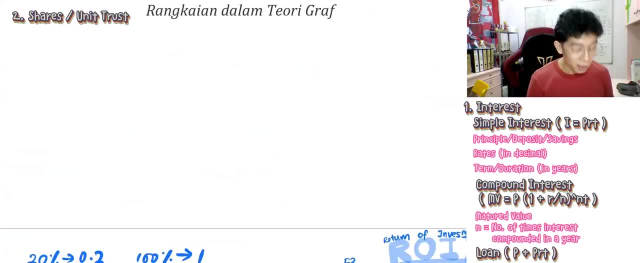 Okay, everybody, the story comes in already. the story It's about cost per unit. okay, where you have to use it in your share-related questions And, ah, simultaneously I will, I will design it into um ROI question as well. 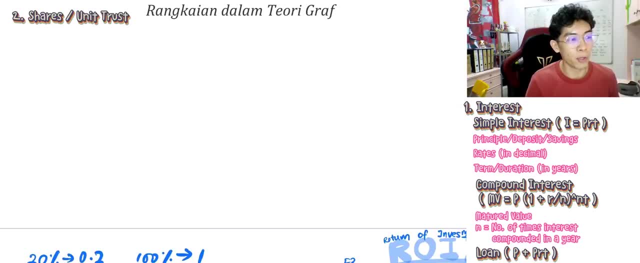 Okay, number one, everyone. if let's say you want to write it, you can write it. If you don't want to write it, just take a calculator and type the answer for me. Ken. really Okay, number one, who is? who is Liang Jie? 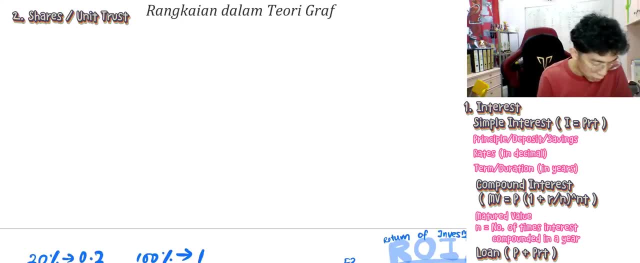 Okay, Liang Jie is not a tutor, Liang Jie is a businessman. Ah, so I write it over here: Liang Jie is a businessman, So story time, story time, ah. So Liang Jie is a businessman. 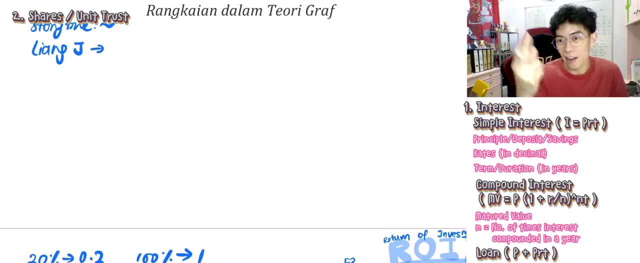 Businessman? okay, businessman, that sells what? Okay, I tell you sell Pilot G2 Pen. Okay, come, everyone tell me: nah sassy your head. Okay, come tell me: Pilot G2 Pen, ah cost how much. 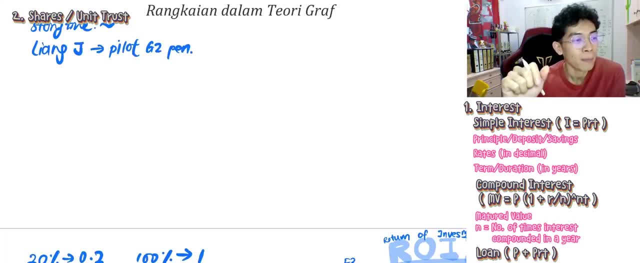 Ah, what's the cheapest price you managed to get before. I don't know now. ah, whether now is like popular among y'all or not, During my year, 20 years ago, right, it's like super popular. 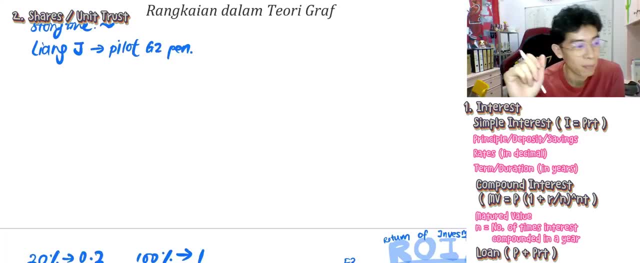 In Form. in Form Form 1, Form 2, up to Form 5, ah, last time Super popular And the cheapest price last time, ah, $4.50.. I don't know now worth how much ah. 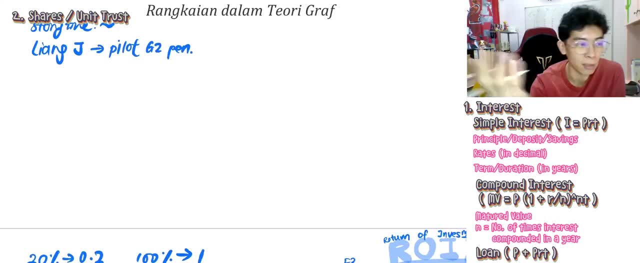 Last time is already $4.50, you know, I think now is around $5, right, I'm not sure. ah, But $4.50, ah is like you have to really go go like quite far to get it, you know. 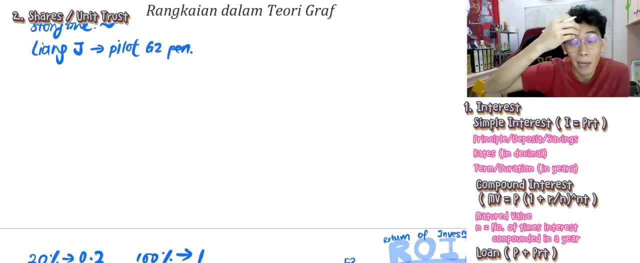 Like last time I go Kedah, only I managed to get this this price, And around here, right, it's like like like $5, $5.20.. Now it's still $5.20, it's like good thing, ah, they didn't inflate, ah. 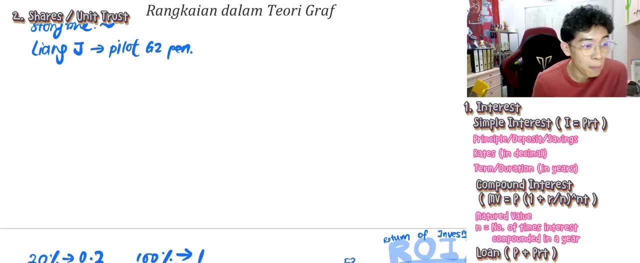 Good, ah, Ah, Eh, Pilot Pen super popular, you know I. I know now, like the Mechanical Pencil, the Shaker Pen is still very popular, But G2 Pen I'm not sure ah. 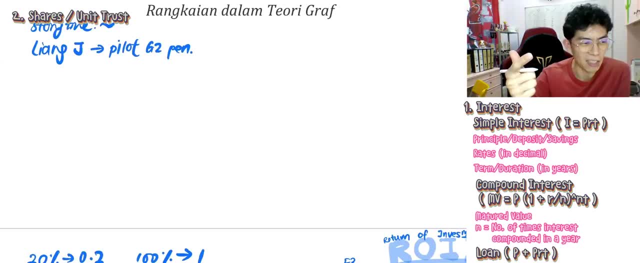 Last time is like G1.. Ah, one more you call like G Tech is there, I don't know, I forget already, But G2 is like super popular G3, cannot. ah, Yeah, okay. 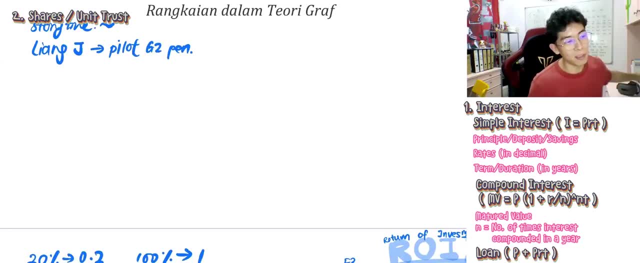 But G2 is like super popular, And now right, because it's like super, super expensive and popular. and I replace it with something else: ah, Pentel, Energel Best, But still expensive. 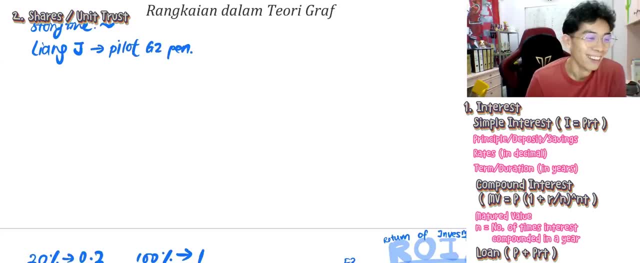 And then after that I use Apple Pen already. Yay, Okay, now come back. Okay, now I'm gonna say: ah, I'm a business man, ah, I'm gonna sell Pilot G2 Pen. We, Eh, ah, Aya, you are. you are new students from which. 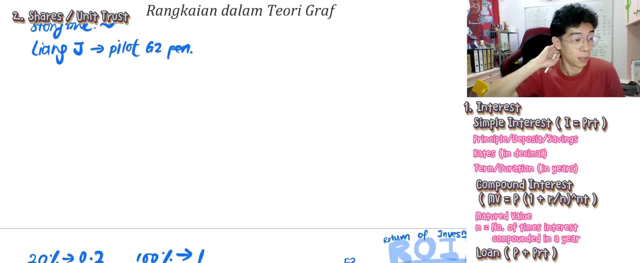 French. You're Gen 9. Do you have this new book, This previous month book? Note, right, Ah, come send me a message 0173817670. later, later, you send to me: Ah, so temporary, you just take a piece of paper and write it first. 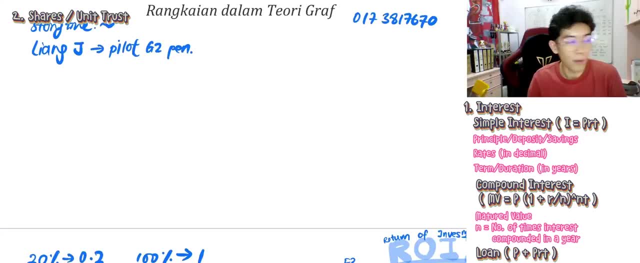 Ah, then I can fly you the PDF. Okay, live, continue, Ah, continue with the, with the story. ah, So I'm a, I'm a, I'm a businessman. Okay, I'm gonna start. uh, I'm gonna little bit faster now. I'm gonna do everything. I'm gonna do everything. I'm gonna do everything. I'm gonna do it. I'm gonna do everything. I'm gonna do everything. I'm gonna do everything. I'm going to do everything. I'm gonna do everything. I'm gonna do everything. I'm gonna do everything. 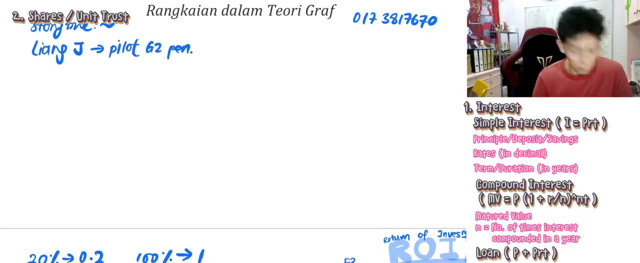 sell pilot g2 pen. so i'm gonna buy a lot of units, probably not. okay, i'm gonna buy 500 units of g2 pen and then eventually sell it. and don't forget, i'm super china, i want to sell profit. later you will see what happened. okay, 500 units, right. okay, because last time, uh, no internet like. 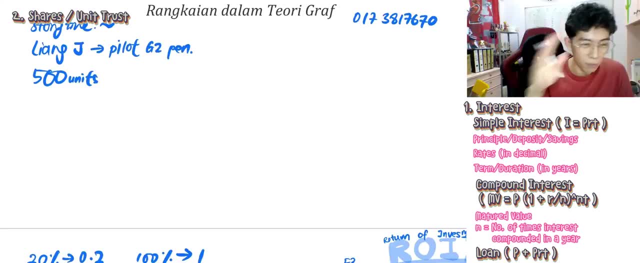 i cannot really contact okay, so i have to travel down to like every shops just to check out all the price so i don't waste my time. so once i go into the the shop, i noticed that the price okay that i buy already. so the first, the first, uh, stationary shop that i go into it's 99 speed. 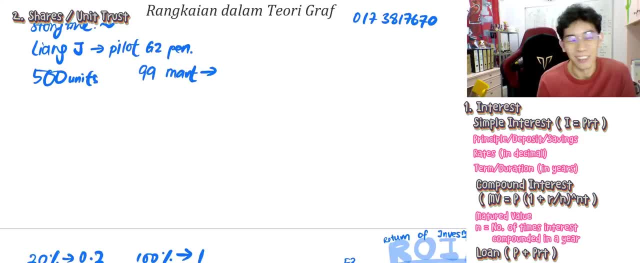 99 speed, but it's not stationary at all. okay, uh, the story you want to copy, or don't copy because it's it's, it's about, um, the idea of cost per unit. uh, then another one is about roi, very easy to understand. okay, so 99 speed mark when i go inside, right, i go inside and check the price. wow, rm firing it. i'm. 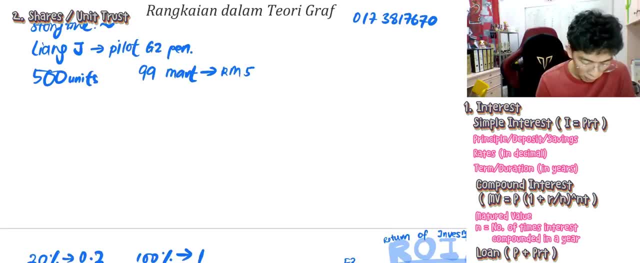 like: okay la, firing it, okay la, buy 100 units la. then then 99 speed mark says what okay la, i got 100 units, i sell to you la. okay, so i just buy it. okay, 100 units. okay, now, after that i say that i need 500, 500 units. right, so i go to another, another uh shop. so i check so that shop is called. 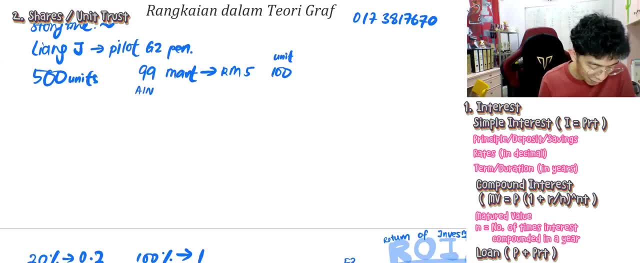 uh, what called? uh, aina, aina stationary, uh, cendrambahat, okay, ssb, okay, aina stationary, cendrambahat. so i go inside and i see aina is there, a aina cheap. a bit la, okay, sell cheaper. so i now say: okay la. 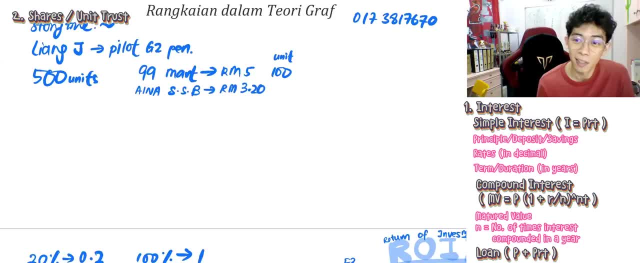 sell cheaper to you, la three ringgit, 20 cents la. so i say, wow, so cheap. ah, hey, you got 400 units or not. i now say, cannot, i still want to do business, man, okay, i sell to you 100 units. okay, la, 150 la. 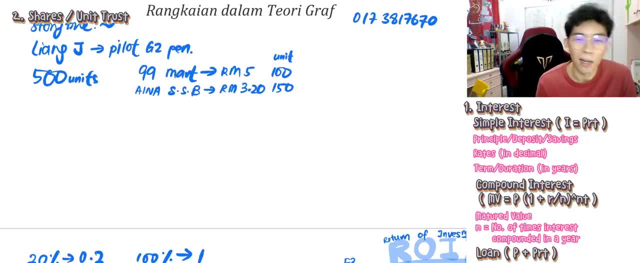 so i take 150 units. then i say okay, good, so i i need another, uh, a few more minutes, a few more units, ah to to complete my 500s. okay, so now i'm gonna go into another one. so i'll go into another shop called hero mart. hero mart like famous, like cheap things, i mean price. okay, cheap price thing. 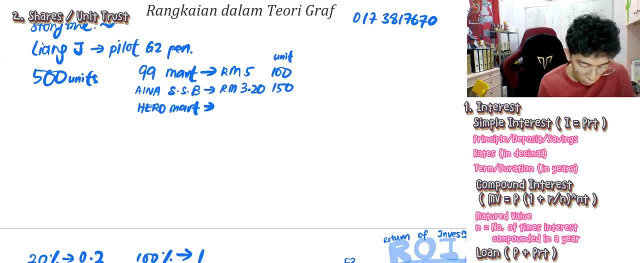 huh. so i go inside. then hero mart says: uh, yeah, i got 100 units there, okay, but i'm selling for 20 cents. so i'll say, okay, la, i take, i take on, okay. so now i'm going to go to another one, so i go into 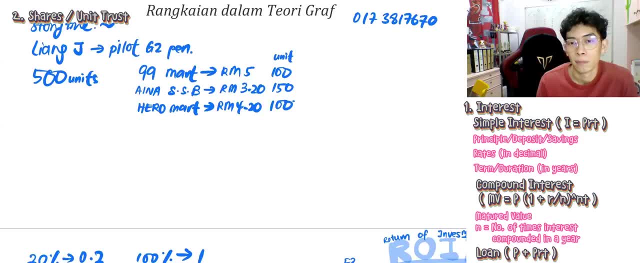 another one. so i'll say: okay, everyone i left how many units i had to buy. i need another 150 units, right, okay, so now i go to the super cheap, one pemborong price, my din. so i go inside. so my didn't say: hey, so happen, i got ngam ngam 150 units or. 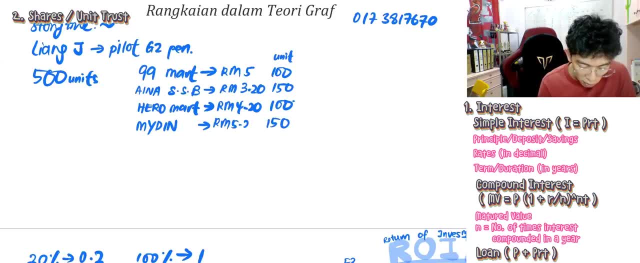 but i sell quite, quite expensive la. find it 20 cent. you want not? i say okay, i don't want travel really take off. okay, now the thing comes in. already i managed to achieve 500 units already. you know what is the average. okay, my question comes in: what is the average cost per unit? 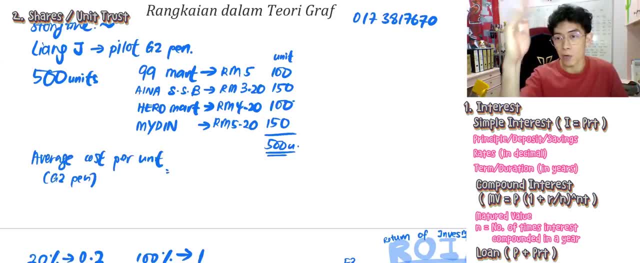 of my g2 pen. okay, come calculate. i want to see anyone do error. i'm going to laugh very loud, super loud. i like i'm going to take my calculator and try it out. oh got one student put 4.4. oh, okay, who put 4.4? come and tell me. i tell you, huh, 4.4. i love very loud and serious. 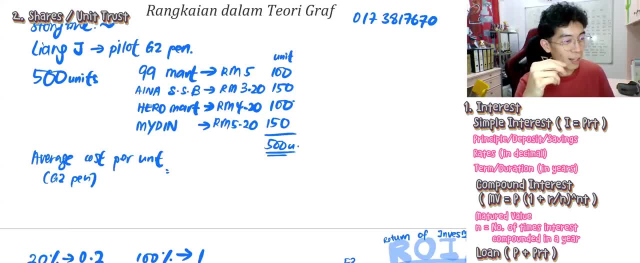 if you get 4.4, you better change. uh, okay, so far, alicia jing and sinru get me: uh, one same answer, but different from the 4.4. okay, come more. so i'm gonna explain a bit. uh, 4.4 answer comes from. 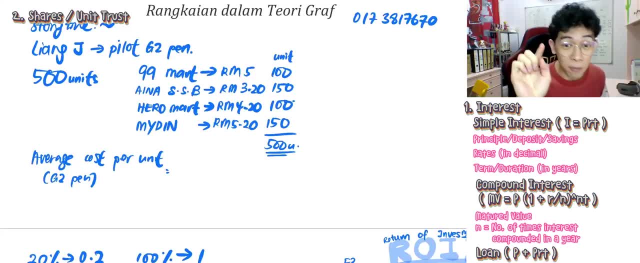 i ringgate plus string, get 20 cents by foreign 20 cents plus 520 cents. these four price you plus together, divided by four, gone. if you do that way, right, provided if all the given units- it's even even meaning- are same, okay, consistent number like 100 units. 100 is 100 hundreds, then can but this one different units. 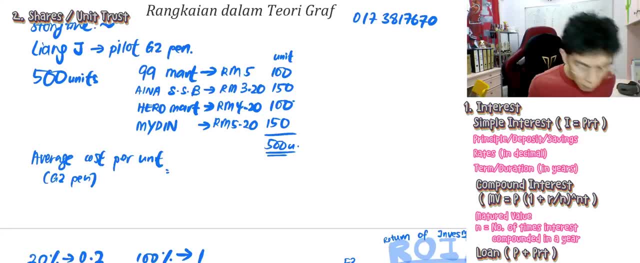 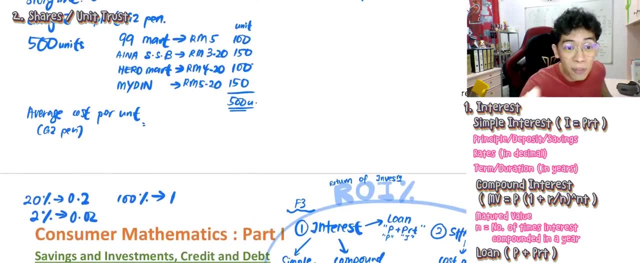 like one is 100 units, the other one is 150, then so on. so the only- not the only- the correct way to handle this average cost per unit is by getting the total amount that i use to purchase all the g2 pens. so i'm gonna add one by one. so i'm gonna add the. 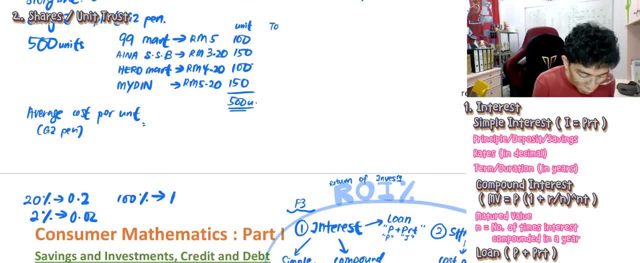 first one: uh, 99, speedmart, the total price. this is the total. uh, okay, the total price, it will be 500. and the other one is like ina, stationary, 300, 320 times uh, 320 cents times 150. now this is 480, this is 420, and the other one is 5.2 times 150 and answer 780. so when you total, 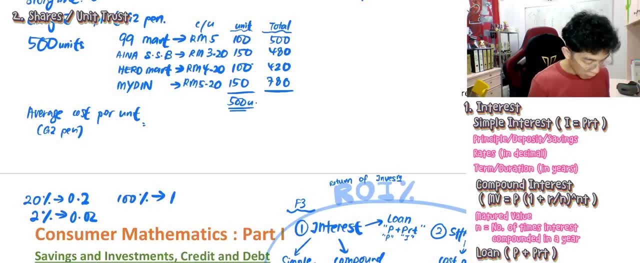 up, right, everyone, the amount that i use to buy everything: 2180, 2180. so now tell me what's the cost per unit: rm2180 divided by 500 units of pen. so you divide by 500 units, your answer is rm4.36 per unit of g2 pen. this is the average cost per unit. so meaning uh. 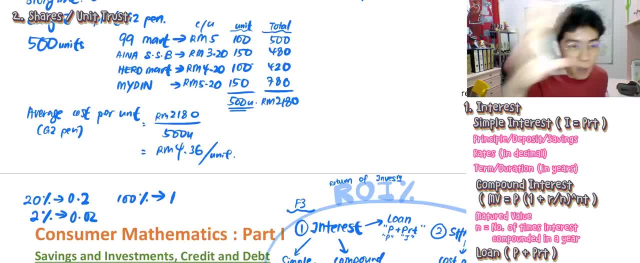 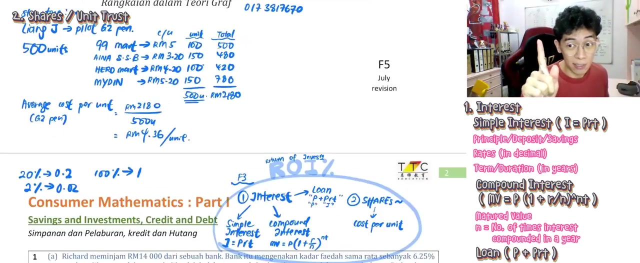 as a businessman point of view. right, the stocks that i have, now all the stocks that i have, uh, per unit of pen will worth foreign 36 cents. ah, so understand the idea of cost per unit, right, yeah, now, so this one you keep it. we straight away hunt down this cost per unit related question. uh, see, ya, now i will come. 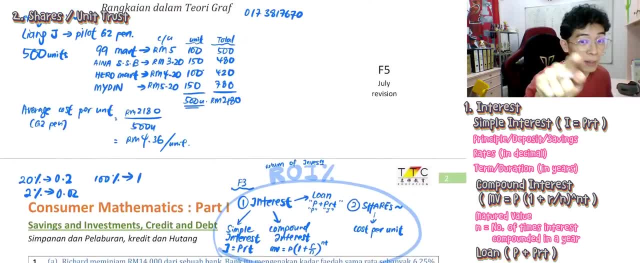 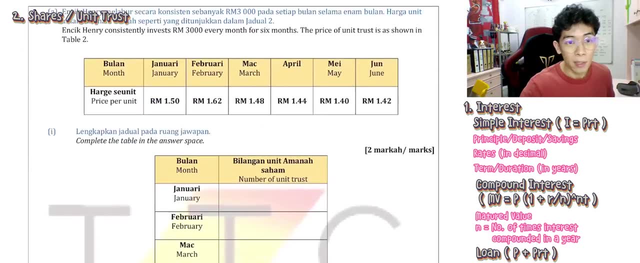 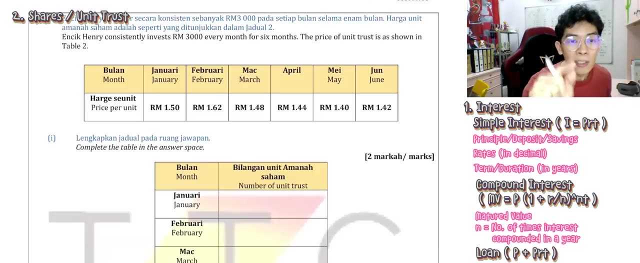 in a while. so let's go into one question. it relates to this cost per unit one. now, everyone, let's move down. uh, let's move down and look at question number three. come question number three. now. i read out: uh, it's about shares, you know, and you have to use this cost per unit related informations. okay, inchit henry. 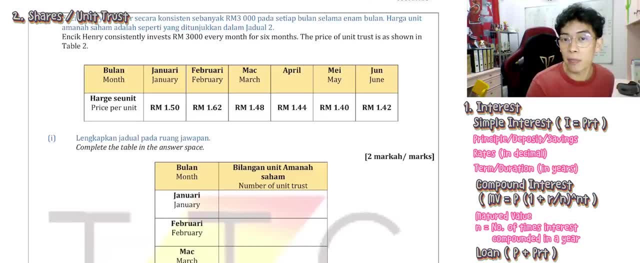 consistently invest 3 000 every month for six months, okay, for six months. every month, 3 000, i repeat, every month: rm 3 000. be careful with the words given and the and the information given. like 3 000, okay, every month for six months. the price of unit trust, everyone unit trust. can you tell me? 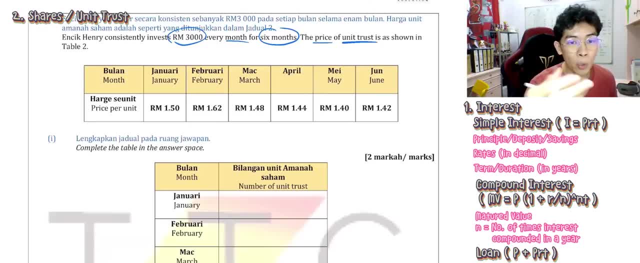 suppose in your syllabus, is the same as what we don't really go into, like the exact definition. we just need to know, like unit trust basically, is the same as what is that word? shares, your shares, okay, but i repeat, uh, in real life, shares and interest, two different things, uh, but they have. 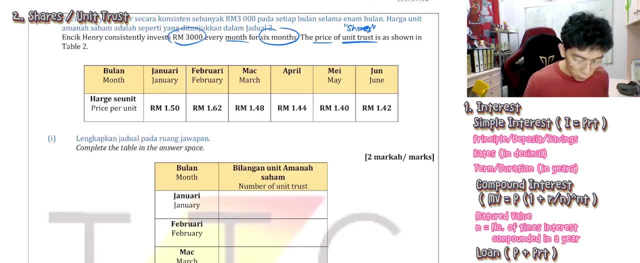 the same function. uh, you, it's for investment purpose. okay, of course, uh, just in depth a bit, you need trust. to be exact, we need to pay, like extra commissions, to the person that manage your funds. okay, shares, you handle yourself. no need, uh, okay, yes, you are right, jinwei. okay, so, uh, but anyhow, they. 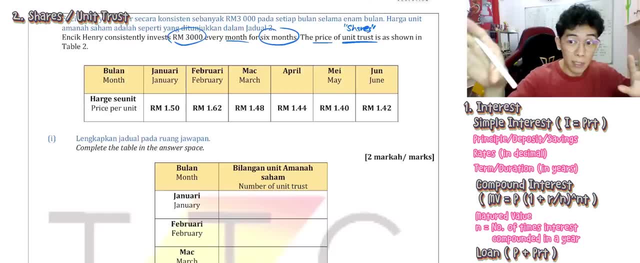 are shares. it says that one manage the professionals. you appoint professionals to manage for you. the other one is that you manage yourself using your own- uh, what's it called share account okay, shares account, okay. so come back then they say that, hey, all the monthly prices, is there, january 150 cent? 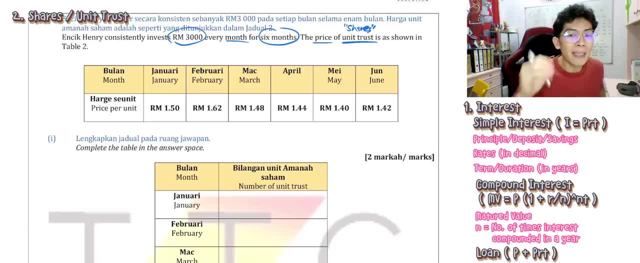 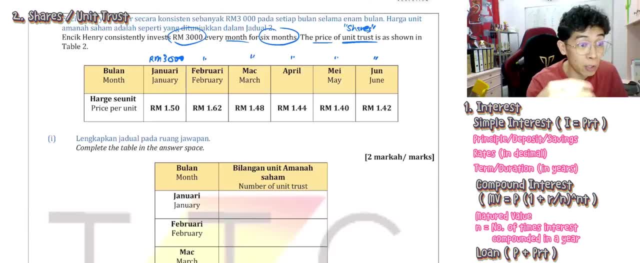 start with c, or maybe sometimes the, the. the strategy start with a. what is that strategy call? of course you are not- uh, i mean, it's in jade, henry, it's not um- applying this concept of throwing all the eggs, or maybe invest all the egg, put all the egg into. 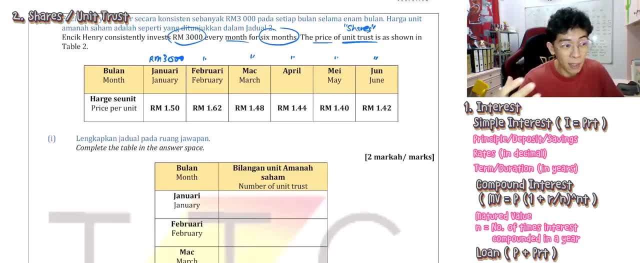 one basket injury. henry is not using this. okay, yes, uh, a very simple way of uh explaining it will be separating your investment, but in your syllabus they mentioned this word: cost averaging strategy. can you write down this one extra one now, just to tell you, uh, in case? uh, they asked? 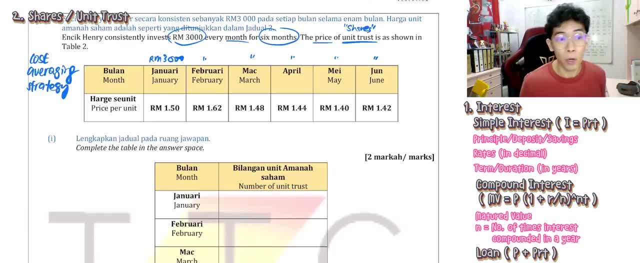 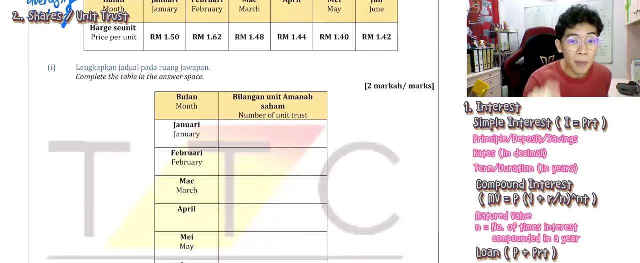 so in jade, henry is applying a method called cost averaging strategy or maybe averaging cost strategy. depends on how, because different book, they have different way of uh presenting the, presenting the, the strategies name: cost averaging, averaging cost. same thing on, okay now. now back to number one. they say: complete the table in the answer space. everybody, january worth one ringgit. 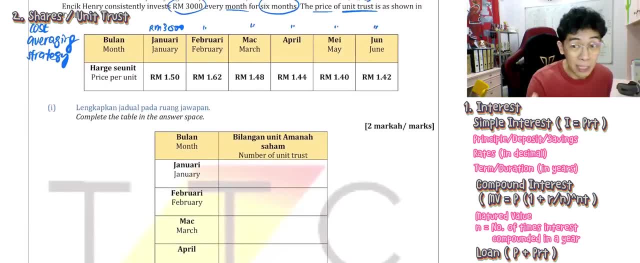 fifty cents right in change, invested $3,000,. how many units of unit trust? or maybe the shares that? Inject Henry, Inject Henry, holding owns okay. Inject Henry, owns Okay, Inject Henry. invest $3,000.. Alicia, thank you. So every unit of shares. 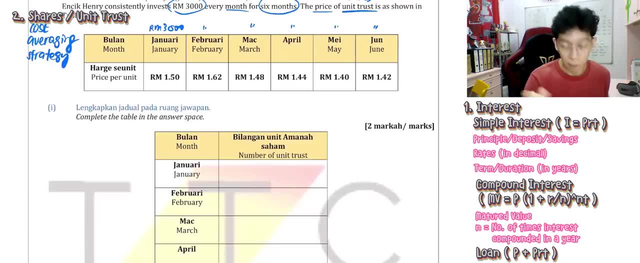 okay, unit trust worth $1.50.. $3,000 as in RM, divided by RM $1.50, the answer is ngam ngam, 2,000 units. So in January, Inject Henry holding 2,000 units of shares unit trust. 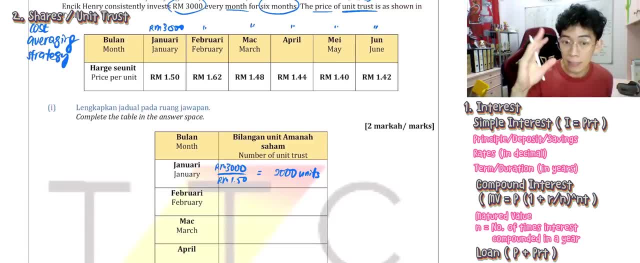 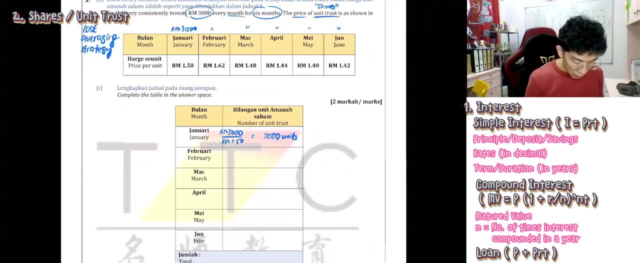 Okay, can you quickly use like one minute, get the rest of the units for me, Like the February, March, April, May, June, come quick, Okay, so I'm going to do it as well. Okay, I'm going to do it as well and see, I'm pretty sure. 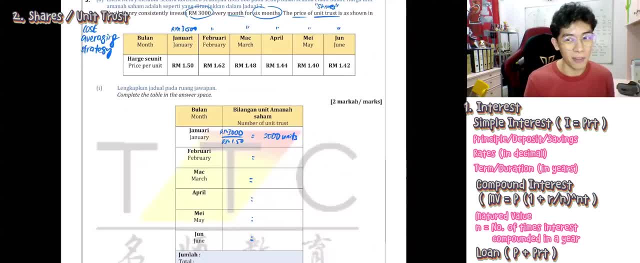 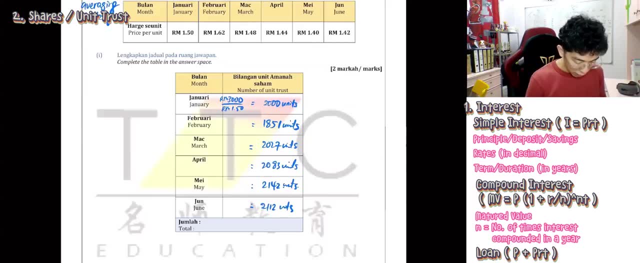 some students will ask me like one very important thing, It's about rounding off. Go ahead, do it first, So eventually I will add up everything. Okay, you check it out as your answer, as compared to my answer. Okay, everybody. 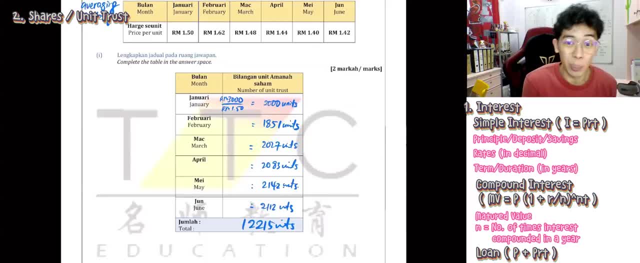 I believe some of the figures. you get something like: I just simply say one of it. Let's say 1851.5,, for example, Do you round off to 1582?? If I say it's like 0.5, 0.7 or 0.8, do you round off? Why? 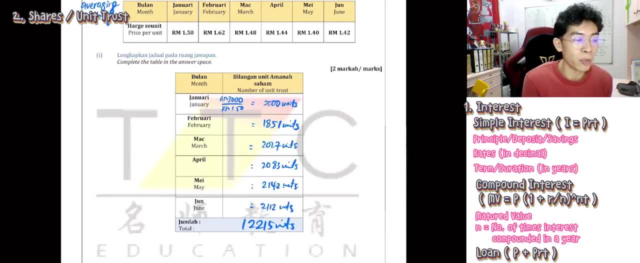 don't you round off the figure? Why don't you round off The reason being you have only a budget of $3,000 per month. $3,000 per month, Okay, $3,000 per month. Do you have extra? maybe a few ringgit, or maybe a few cents? I'm not sure. 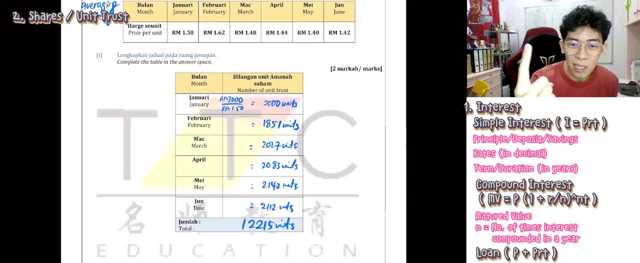 about it to buy that extra one unit? You already say you're going to budget $3,000.. Why are you going to extra? pay it right? That's the reason. Okay, so that's why you can't even afford another. 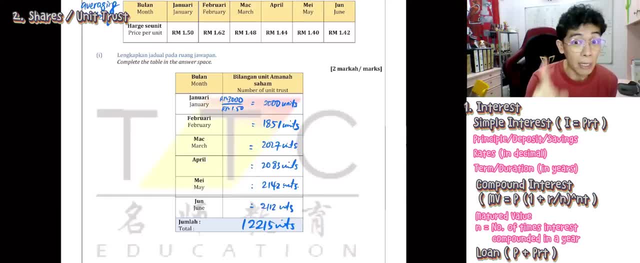 extra to buy it because you budgeted $3,000 for it. Understand that, Although some of you might say teacher, $3,000 only, Okay, so I will say $3,000 for some people is also quite you know. so you cannot say like this: So how if the figure I changed to $3,000,000 gone right? 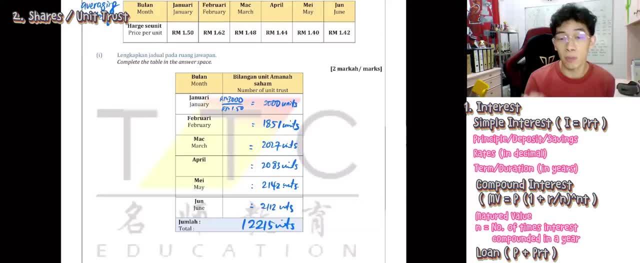 So cannot say like this: So that's why you have to ngam ngam. So if I say extra by point, something you cannot round off as well because you can't afford that extra. Okay, because of the figure given. So because you're budgeted $3,000.. So cannot simply do that. Okay now. so now you know. 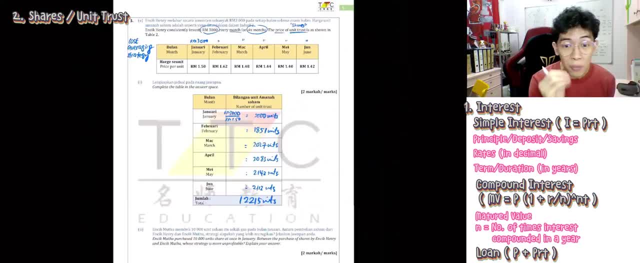 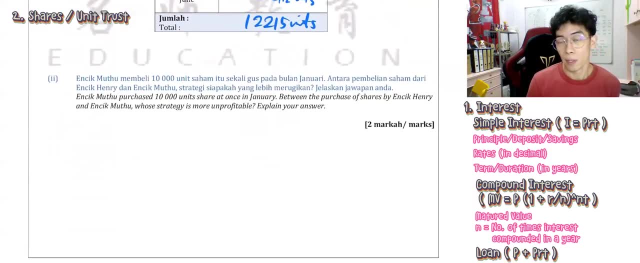 that Inche Henry owns 12215 units of shares. Okay now. now the second question comes in. Who's the second person? Inche Mutu, Everyone. two seconds silent. We're going to separate, nicely, Don't read, don't read. 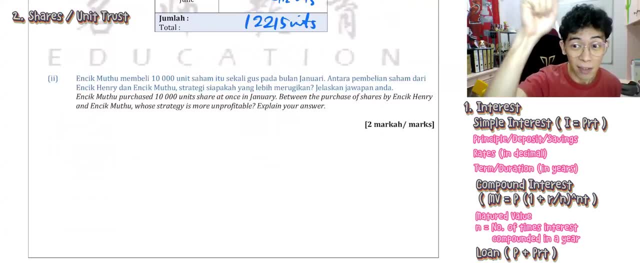 Don't, don't, don't mix up the names. you know, just now it's Inche Henry. This one is Inche Mutu. Okay, Inche Henry applied cost averaging strategy to spread out the investment to six months. you know, every month $3,000.. But Inche Mutu purchased 10,000 unit shares. 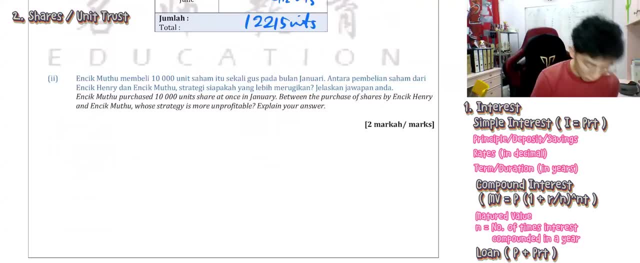 once in January. This is called lump sum purchase. This is called lump sum purchase. Okay, one lump sum purchase. Okay, invest everything, throw everything into one basket. Okay, So everyone. can you tell me, January, how much is the price? Yes, you're right. 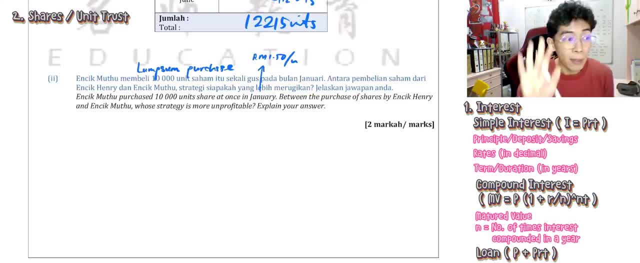 January is RM1.50 per unit. Now listen carefully. Agree or not. Inche Mutu's cost per unit is exactly $1.50.. So Inche Mutu's cost per unit is exactly $1.50.. So Inche Mutu's cost per unit is exactly $1.50. 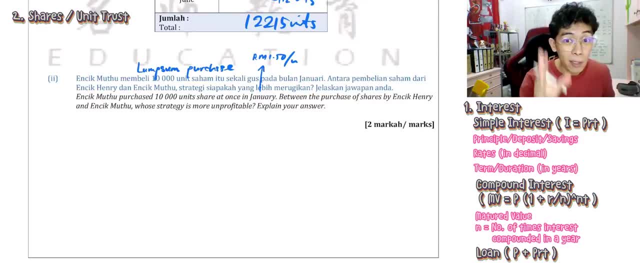 Okay, I repeat, Inche Henry's cost per unit for the unit trust, or maybe share, is RM1.50.. Obviously, because one lump sum purchase, the price fixed already RM1.50.. Okay, Just like if I mentioned my G2 situation, let's say I didn't go any other place. I just go to Aina's stationery shop I say 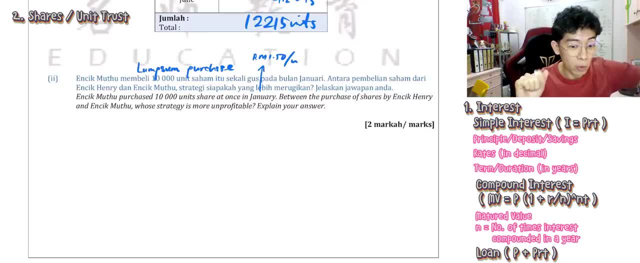 Aina, please sell everything to me. Sell everything to me- RM4.20.. RM5.00 units, So my cost per unit will be RM4.20.. But what happened is I choose to spread out. I choose to spread out right, So that will be cost averaging. So can you see the G2 situation? 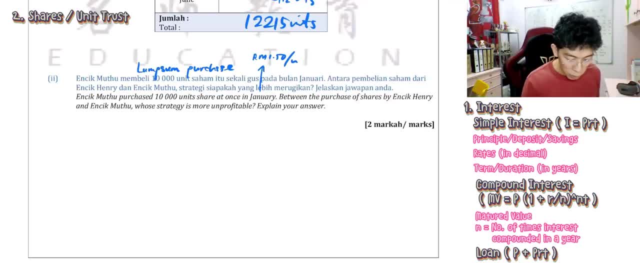 is the same thing. Yeah, So now, between the purchase of shares by Inche Henry and Inche Mutu, whose strategy is more unprofitable? Whose one is more not worthy? That's the meaning. Explain your answer. Explanation will be in calculation format. 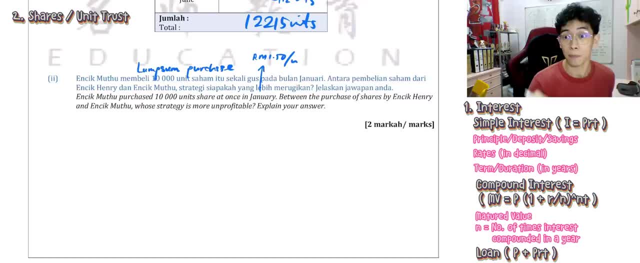 And I will be using cost per unit to prove. So let me write Inche Mutu first. So Inche Mutu: very obvious already, You don't have to even do any calculation. The cost per unit is RM1.50 per unit. Okay, Per unit. So how about Inche Henry, Everyone Inche Henry. cost per unit. 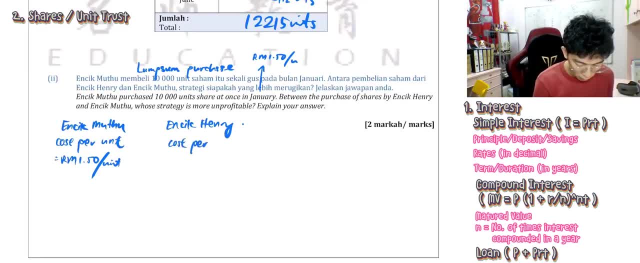 how much Inche Henry cost per unit, how much Number one. remember my G2 situation. I get my total cost, The total amount that I used to buy all the G2 pens: 500 unit of G2 pens And same applies. 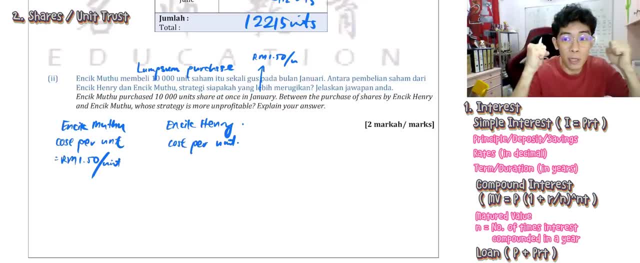 here You have to get the total investment value that Inche Henry used to purchase all the shares. So what is the total amount that Inche Henry used to purchase all the shares? What's that price? Every month, 3,000 for six months. Jinwei, thank you, 18,000.. So 18,000. 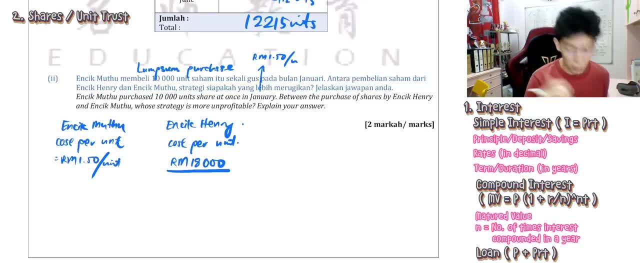 divided by how many units of shares Inche Henry owns 1,, 2, 2, 1, 5 units per unit. So can you see it's RM per unit, cost per unit: Saw that or not? 1, 8, 0, 0, 0 divided by 1, 2, 2, 1, 5.. 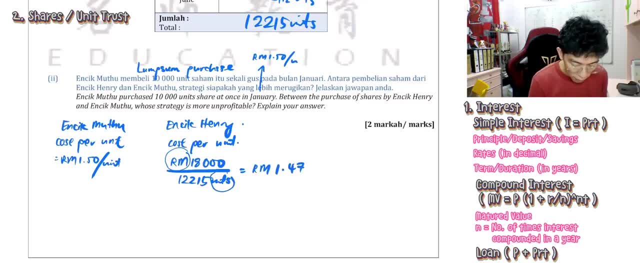 Your answer is RM1.50 per unit. So how about Inche Henry? How about Inche Henry? How about Inche Henry? Your answer is RM1.47 per unit of shares. So everyone. can you tell me now whose one is not? 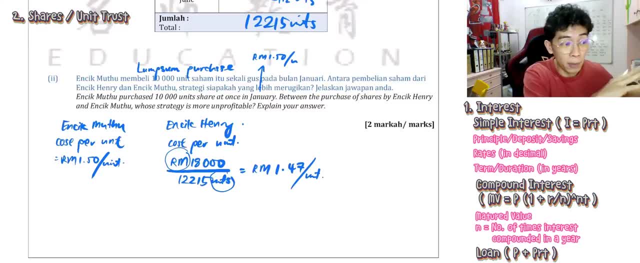 so profitable- Unprofitable in this case, Obviously Inche Henry's one. Why? Because Inche Henry purchased the share RM1.50.. RM1.50.. Okay, So I repeat the answer, The answer you will write. therefore, you write it yourself. Therefore. 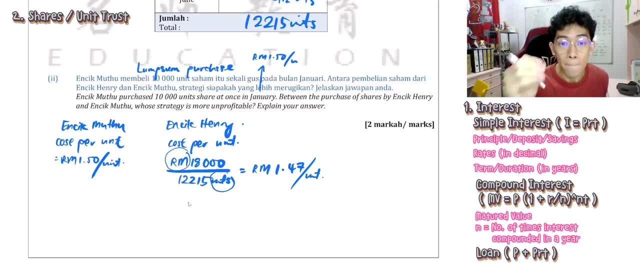 Inche Mutu's strategy is more unprofitable And of course, the explanation, it's the calculation above. Okay, Now, so everyone, now, let's go to ROI, Let's go to ROI. So I go up, go up. 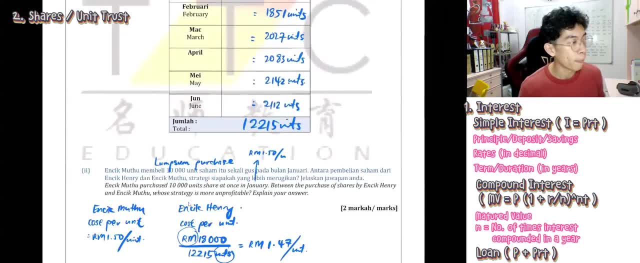 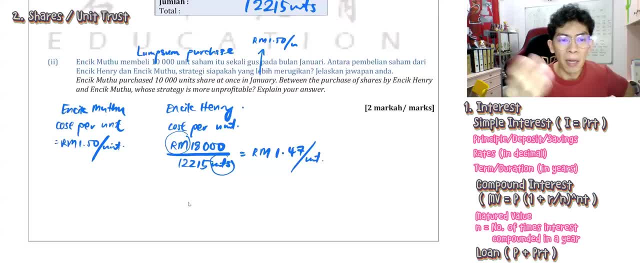 ask me to ask me about it, teacher. But a bit not fair. Inche Mutu, Inche Mutu, total investment is only RM15,000. And Inche Henry is RM18,000. And, moreover, the unit's owner. 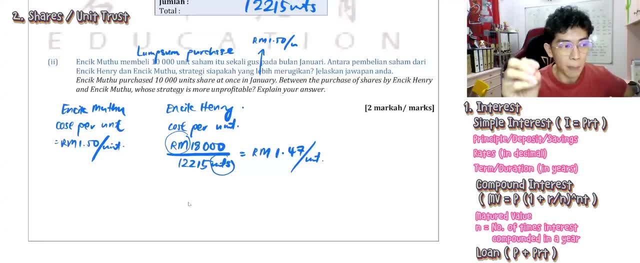 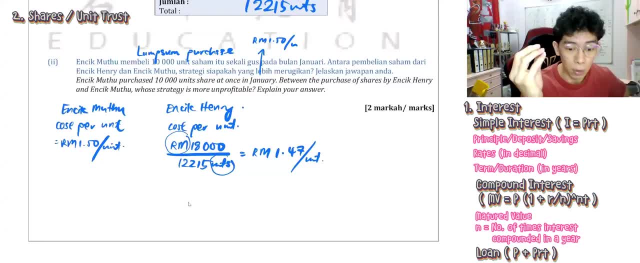 Mutu Inche, Mutu Total, you can see it's like RM15,000 only, right. So we restrict to the budget and by using the budgets to calculate the average price per unit to compare the sum. So we are comparing using the limited budget. So, anyhow, when you compare stuff, 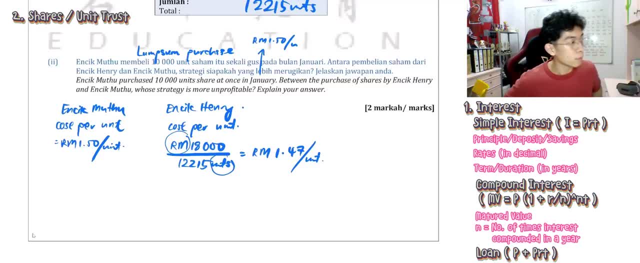 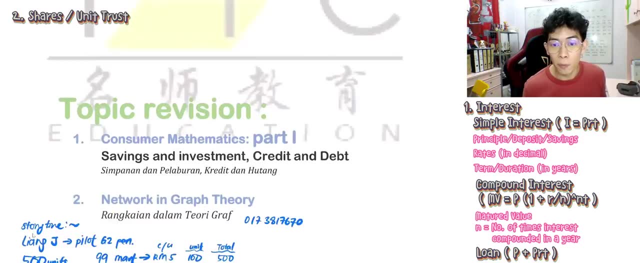 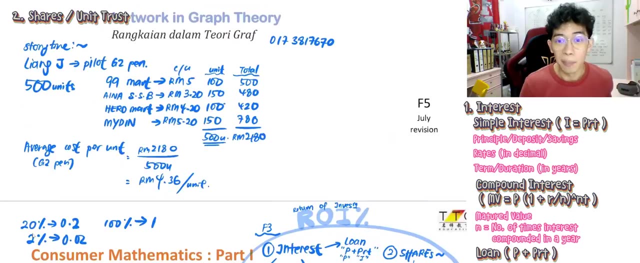 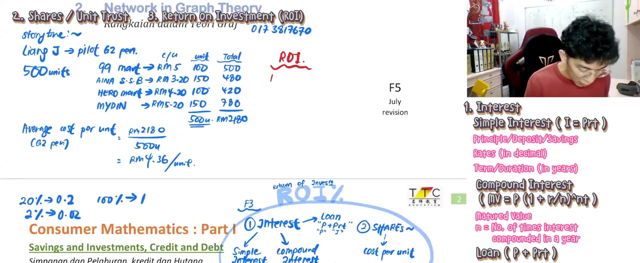 right, you go back to the, to the budget. Okay, Yeah. So everybody, everybody, we will go back to the, to the information above. Okay, Information above. And now I'm going to go up to the business. okay, now i'm gonna talk about roi. okay, roi. my cost per unit of the g2 pen in my in. 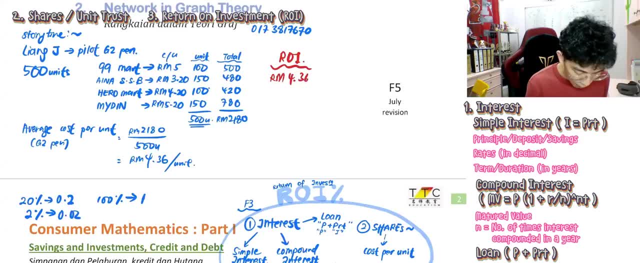 my storeroom, my stock foreign gate: 36 per unit. okay, that's my, that's my cost, cost or maybe the original price and i say, just like very cheap, i want super profit. so i say that i'm gonna sell it. okay, my selling price come. my selling price: rm. 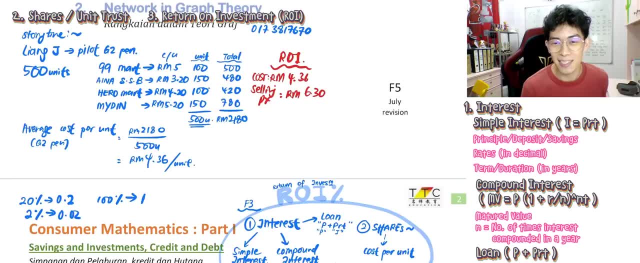 six ringgit 30 cents. i want y'all to try it out. try to get me your roi return on investment in percentage come right. so while you're doing your roi, right when you're trying it out. so, like what i mentioned, try to get me your roi return on investment in percentage. 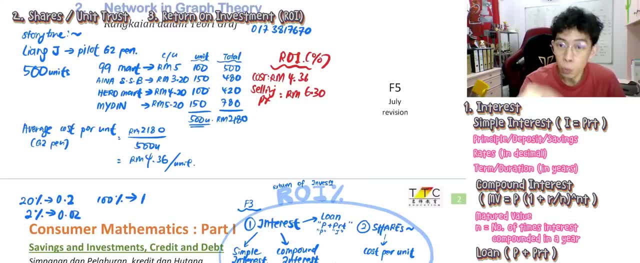 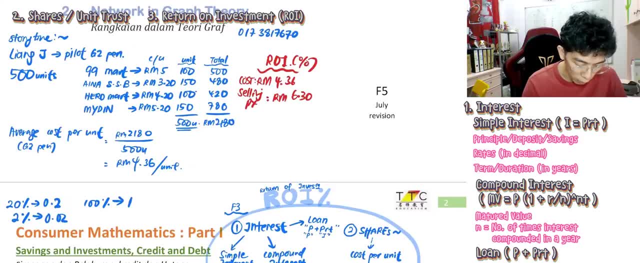 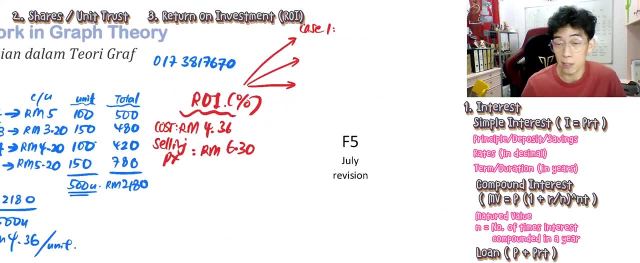 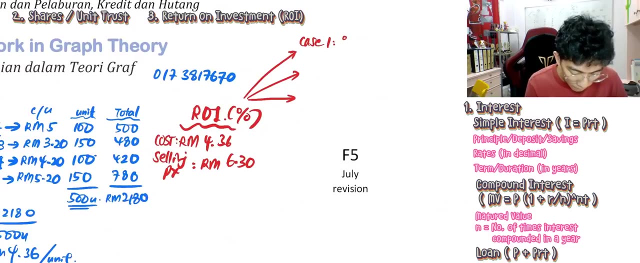 trying it before, okay, so while you're doing right, uh, while you're doing halfway right, so i'm gonna say: right, it can be, it can be, it can be, uh. interpreted in in three different cases. case number one: roi- return on investment is the same as percentage of profit. 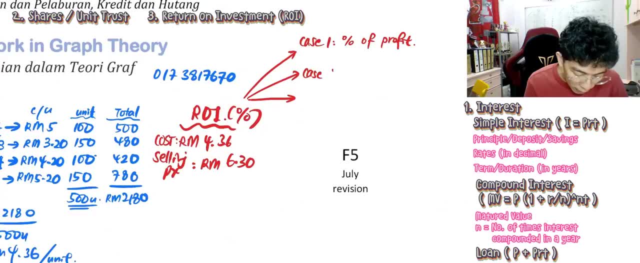 it's the same thing. roi is the same as percentage of increase in price, in price, okay. roi is also the same as okay. roi is also the same as percentage of um. return basically means percentage of return of investment, okay, and return, you know it will be something that you gain, okay, something that you gain, uh, your bonus, your dividend. 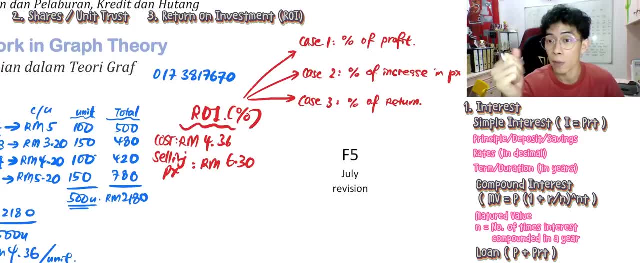 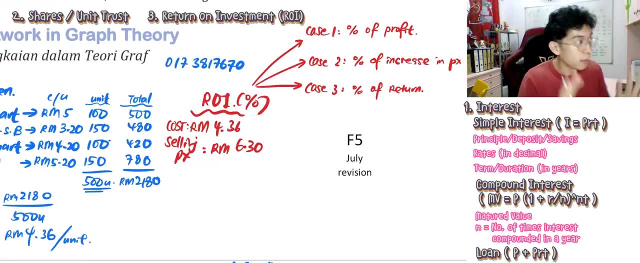 everything like whatever, whatever things that you gain are your profits, okay now. so now let me interpret it for you. is here now, everyone see in, in in business and man point of view are, let's say, from my point of view, instead of referring it as an investment, i refer it as a. 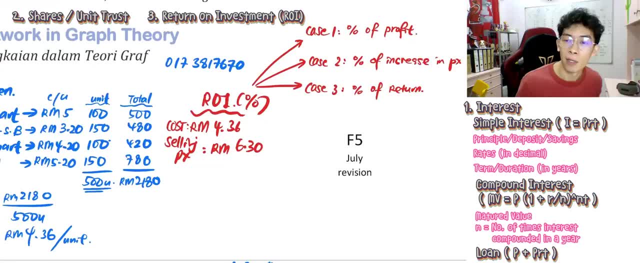 percentage of profit to my, to my partners. so i tell them our percentage of profit for g2 pener, g2 pen, the profit, the profit inside here, obviously it will be how much time? tell me what's the profit? um, let me calculate using per unit. okay, you want to use totals? okay, now run. uh, so, like a number of, 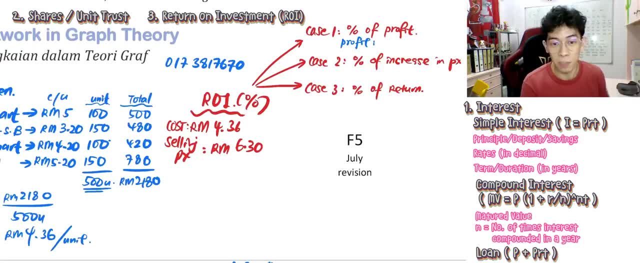 So, like Aina is using total right, I'll be using per unit. I'll be using per unit. Okay so, RM6.30 minus RM4.36 per unit, My profit is RM1.94.. Crying out. 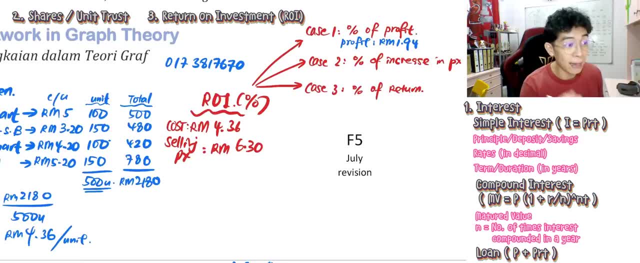 RM1.94.. Of course, if you times with 500, then you'll get RM970.. That will be the total. It's the same thing. don't worry, It's the same thing. Okay now. So I'm using per unit. 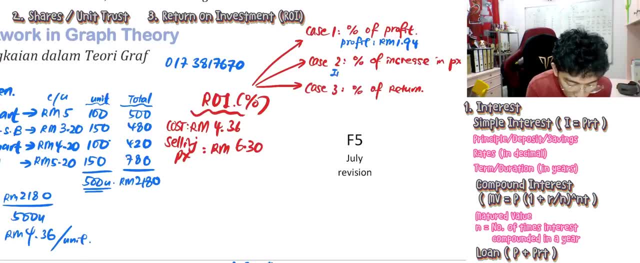 Then if I say: what is the increase in price? Increase, Oops, The increase in price. It's the same thing Crying out: What is the return per unit? The return per unit. The return per unit is also RM1.94.. 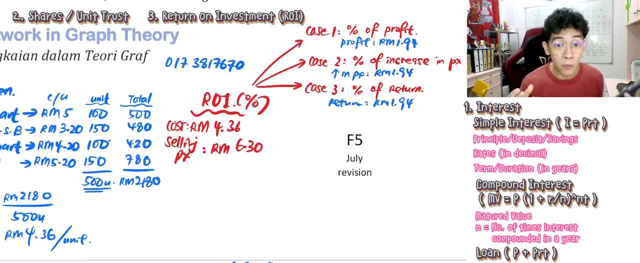 Crying out. So, do you notice, in order to get a percentage for all these things you get to, you need to what You need to do the same thing. You need to do the same thing: 1.94,, which is the. 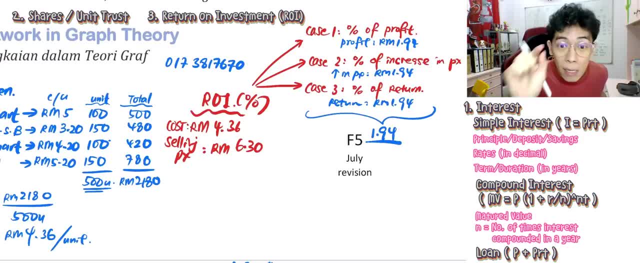 I forgot. You want written on investment actual formula. It's initial. sorry, It's your total return. The original formula is the same as this one. Okay, Divide by initial investment, Initial investment times 100% And your total return: RM1.94 for one unit. 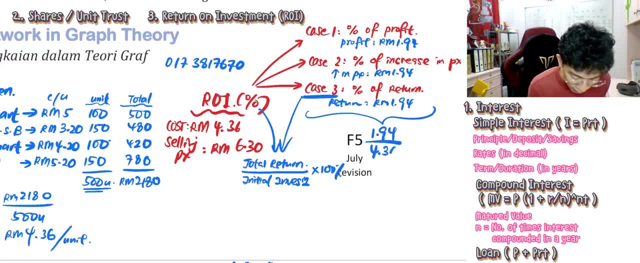 And then divide by the original price: RM4.36.. If let's say you are using total, you will put 2180. Times with 100%, Divide by 4.36 times 100%. RM1.94 divided by 4.36 times 100%. 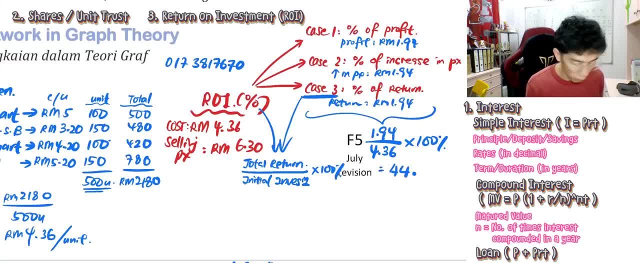 Your answer is 44.5%. So my return on investment- either you say total or maybe per unit- it's the same answer- It's 44.5%, 0.5% for my G2.. So is this investment worthwhile everyone? 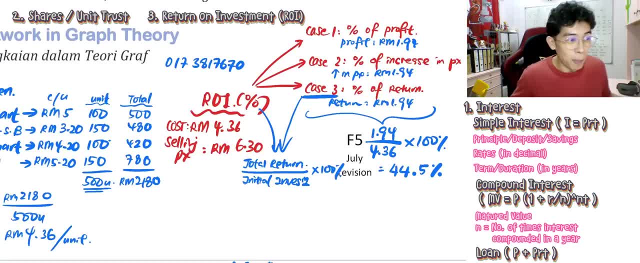 Is the percentage high enough or not? It depends on how you interpret it. Depends on how you interpret it. Now I tell you something everyone Agree or not. you think about it before you answer me. Agree or not, actually? 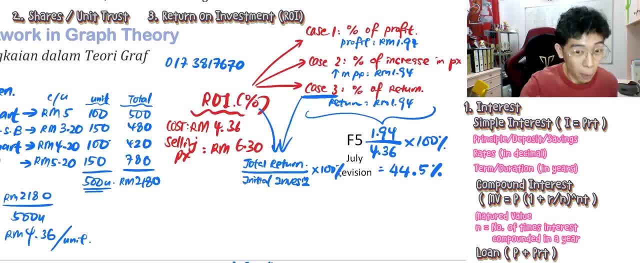 your interest rate from your fixed deposit. it's also return on investment. You get what I mean. And do you notice? why not I check instantly for you? Okay, let's check it now. Today is like August, 4th of August, right? 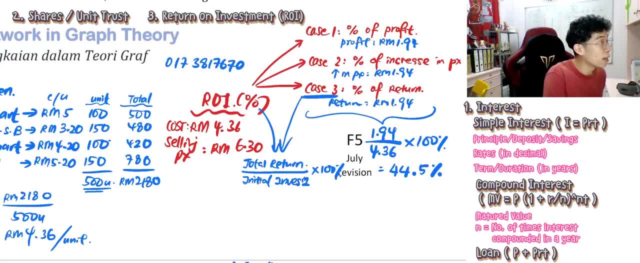 2021.. Let's see our fixed deposit interest rate. Our fixed deposit interest rate, how much is it? Let's see our fixed deposit interest rate 2021.. Wow, best Everyone, what I see from Google so far, I see. 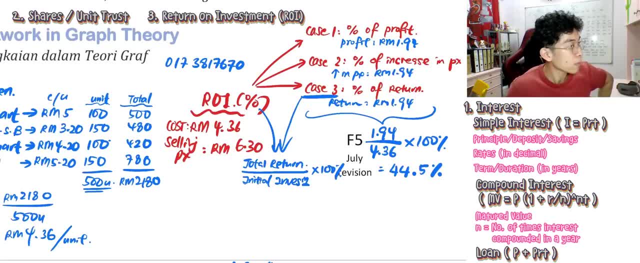 okay, the first one I see here is like RHB, RHB Bank. the FD best rate for 12 months: 2.5%. 2.5% for one month, Per Gila. Okay, then imagine if you sell G2Pen. 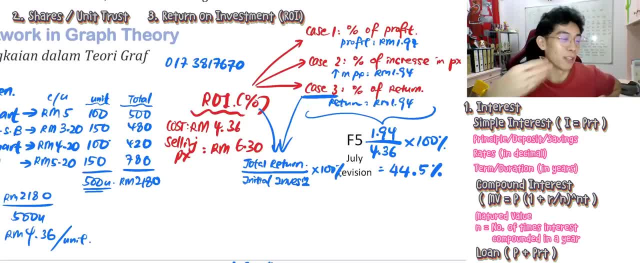 but of course you have to do some marketing. You have to sell to your friend- hey, you want to buy G2Pen or not? So you get. you need to work a bit, So you get 44.5%. Which one you want? 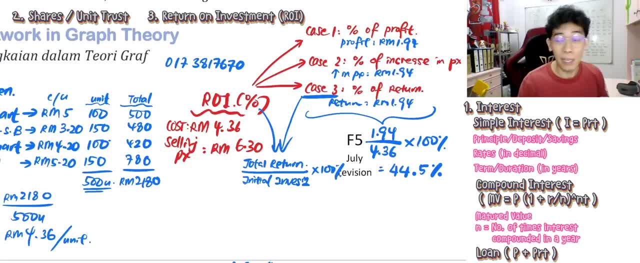 So see what you want. Okay, so that will be the return on investment. So see how you interpret it. Because ROI is a general stuff, It can be ROI in your property amount. So let's say I buy this property. let's say: 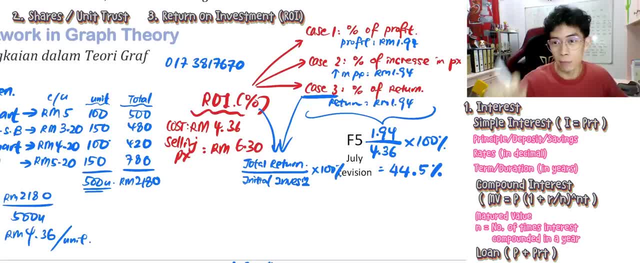 I buy the house that I want to buy. I buy the house that I'm staying now for 500,000.. And 10 years later, 10 years later, 10 years later- right, I'm going to sell it at 1 million. 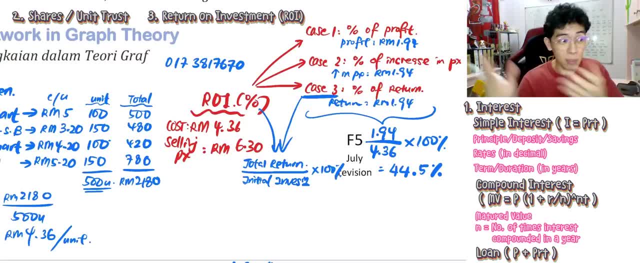 So what is the ROI? You get the difference, then divide by 500,000, then times 100%, then you'll get it. So the ROI is 100%. Okay, got it, But you have to know. after 10 years you know. 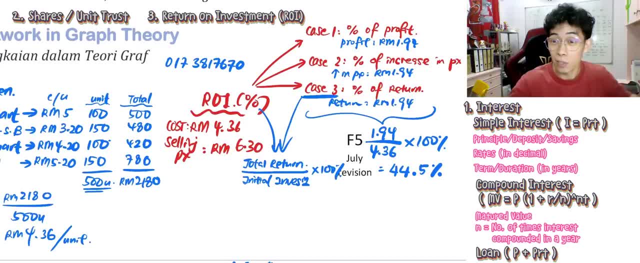 So the 10 years you divide by what You divide by 10 years, So per year 10%. So it depends on how you interpret it. So imagine if let's say you sell G2 Pen. you consistently sell it every month. 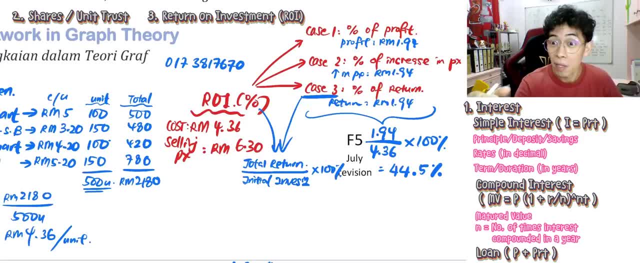 So you return 44.5%. 44.5%- Wow, nice. Okay, so see how you look at it. So another one will be: your ROI can be more than 100%. You don't tell me your gain. you want to restrict in 100%. 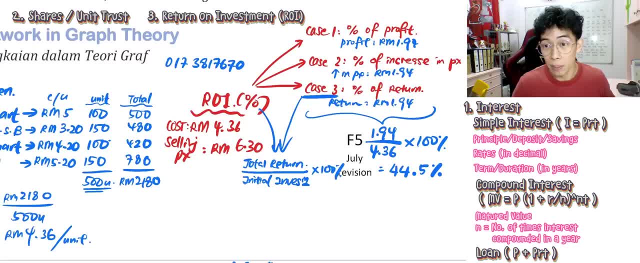 So what do you earn? Your return on investment percentage. it can be 1,000%, It can be 2,000%. So see how you market it. Okay, got it. We try ROI now. We try ROI now. Okay, everybody. 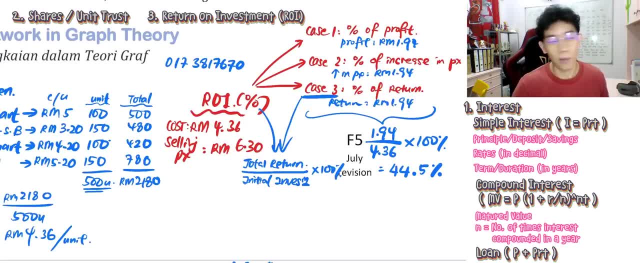 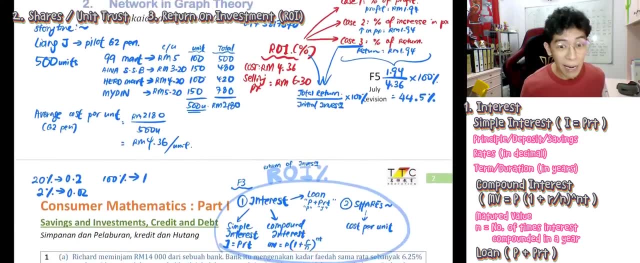 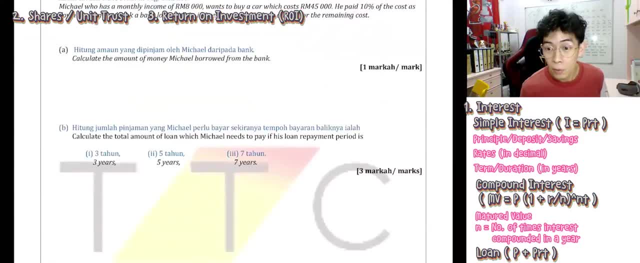 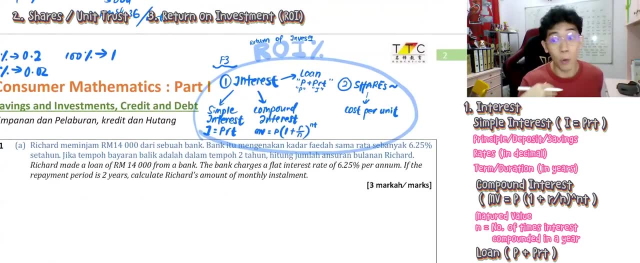 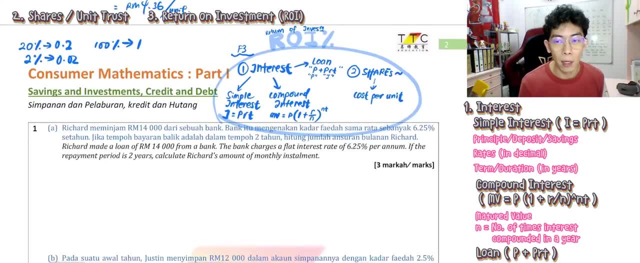 Okay, Come Question number one. Richard made a loan, Oh, made a loan of 14,000 from the bank. Tell me the initial 14,000 stands for what. Just tell me the first alphabet can read it: 14,000 is the P. 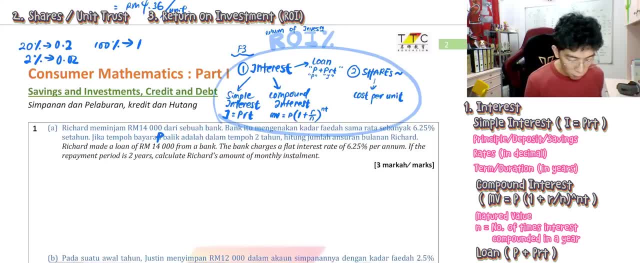 Yes, the principal, The bank, charges a flat rate. Flat means simple, Not simple as in the question, simple as in the formula, But not simple as in the question. simple as in the formula, As in the formula, As in the formula, it's about simple interest. 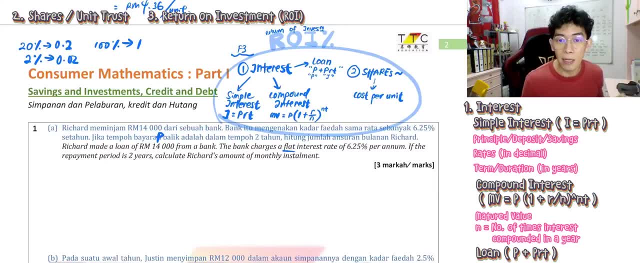 Flat interest rate of 6.25 per annum. Per annum means per year, Then 6.25, nobody put 6.25 over 100. We put 0.0625.. If the repayment period is two years, hey, repayment period two years. 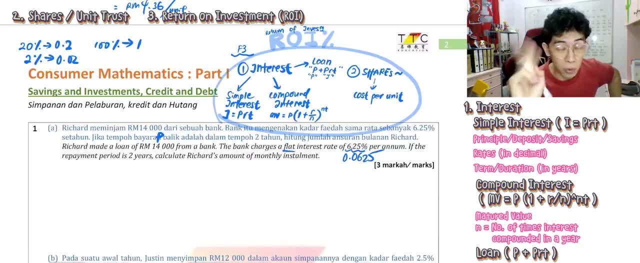 means your loan. it's for two years on, you know. So your interest. you're gonna calculate two years, Calculate richest amount of monthly installment. Okay, the monthly installment, we leave it first. Let's get the total loan that you're gonna repay to bank. 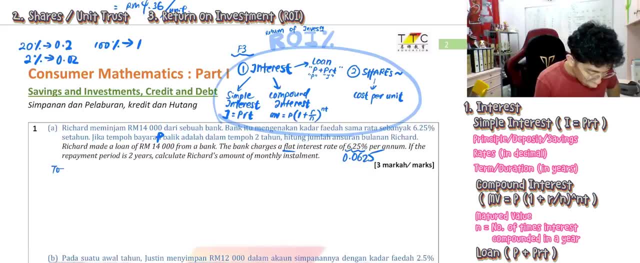 including interest on. So your total loan including interest, including interest, or maybe the total repayment of the loaner, it will be P plus PRT, 14,000 plus with 14,000 times with 0.0625 times with two. 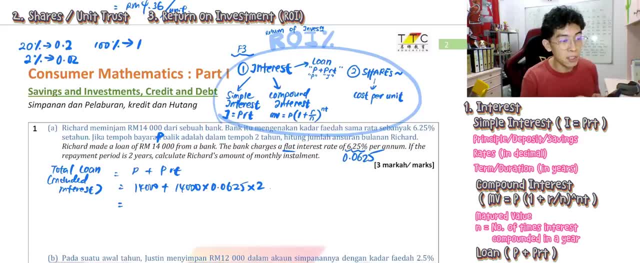 Get me the final figure. come quick, Jingxian. remember to always put 0.0625.. We have to slowly use to the decimal. Yeah, So it will be 14,000.. So it will be 15,000. 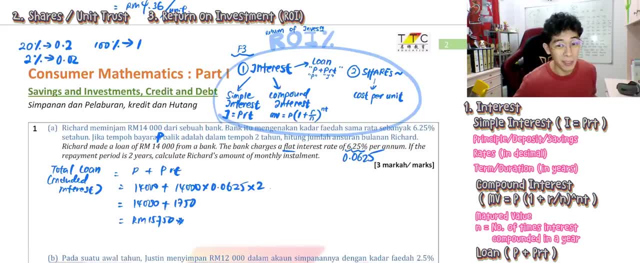 Scare me, Aina. I think you actually put 0.625.. You missed out the zero because I did that error also. You try and see: Okay, this is the The total repay back to the bank. You don't. 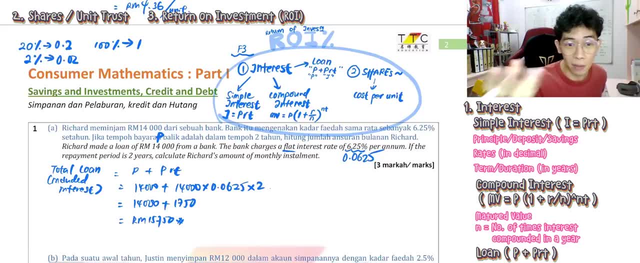 You cannot say like bank, You pinjam 14,000 from bank, then you pay back bank 14,000.. Not fair, ma Bank pinjam you money wo, But they charge interest very high. la Sad, They give you little interest. 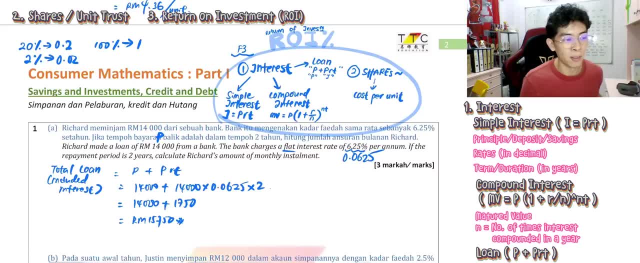 like fixed deposit, 2.5%, but this one they give you year. Okay, so the next one, the next one: the repayment period is two years, everyone Two years. ah, Two years equivalent to how many months? Okay, 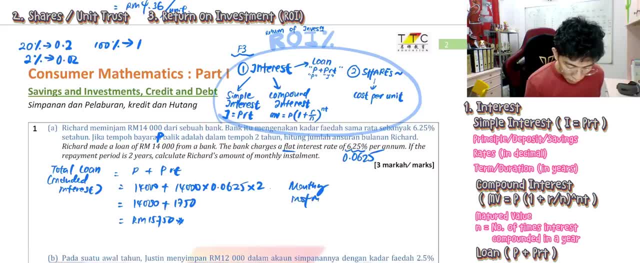 So this is my monthly instalment. My monthly instalment it will be 15750 divided by 24.. Thank you, Divided by 24.. So per month you have to repay 656.25.. So that's the per month. 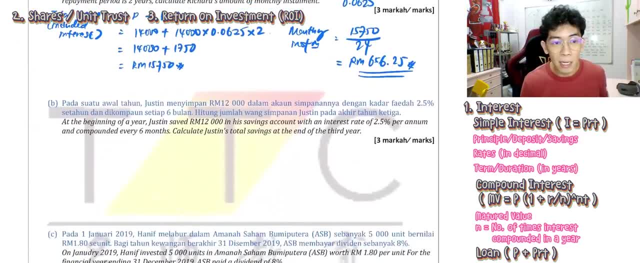 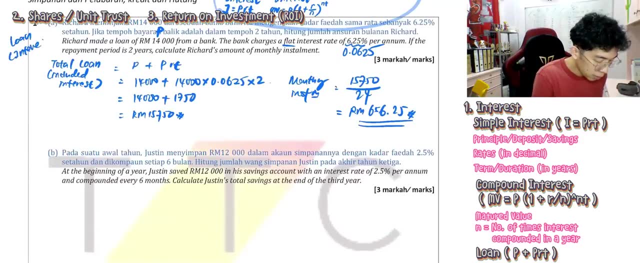 Okay, per month figure. Okay, come quick. Next, next Question B. Question B: This one is about loan, ah, Loan, and it's about interest. Okay, it's about the repayment period. ah, as for as for monthly and. 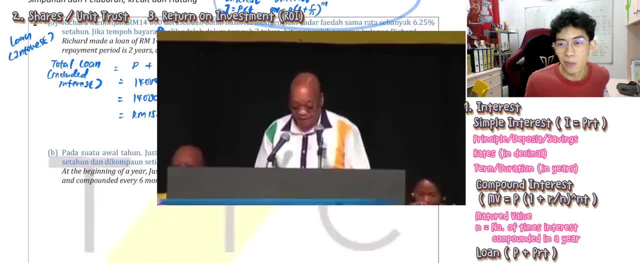 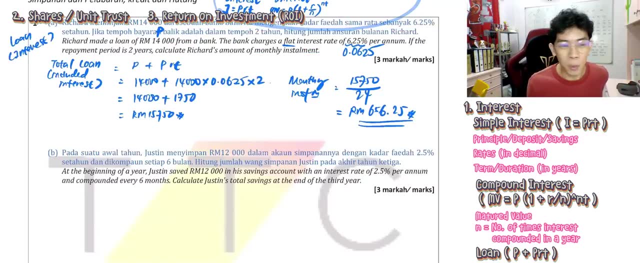 Okay, P At the beginning, In the beginning, Beginning of In the Justin save 12,000.. Eh, what is 12,000? come Initial initial like Yes, correct, Okay, correct. That's the initial P principle. 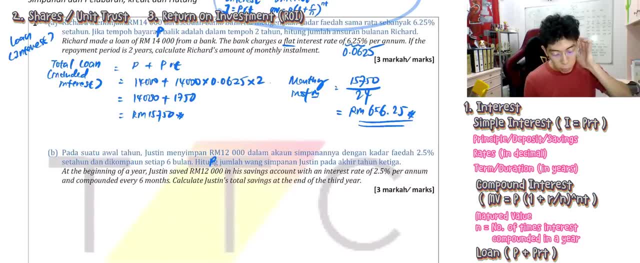 Okay, principle In the savings account with an interest rate of a 0.025, nobody going to see that one, Be careful ah. per annum. Sometimes they nothing to do, They try to like purposely con you ah. 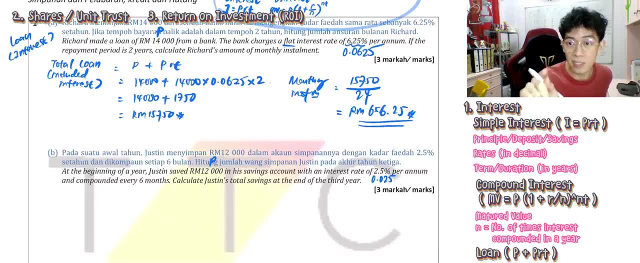 They put per month and gone: Ah, so norm. ah, you have to check what is that. But normally they put per annum, one ah. Per annum means per year And oh, everyone compounded every six months. I sent a YouTube link to to everybody. 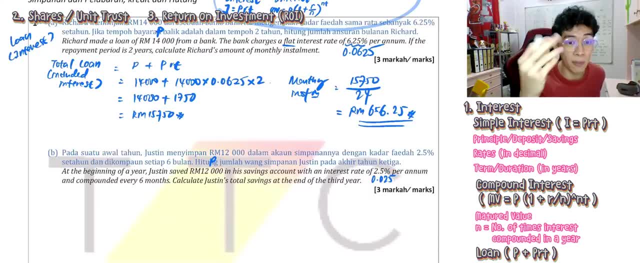 You can see that That's about compound interest, Ah, so in case you need more further explanation, you can look at that. Ah, I sent you the link there already. Okay, compounded every six month. Everyone, look at the formula. 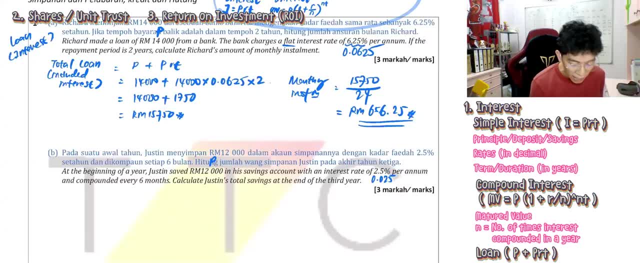 Calculate, Justin, total savings at the at the end of the third year. So it means the total investment, the FD. ah, it's three years. MV matured value equals to principle One plus R over N, then NT. Let's put all the relevant info that you know first. 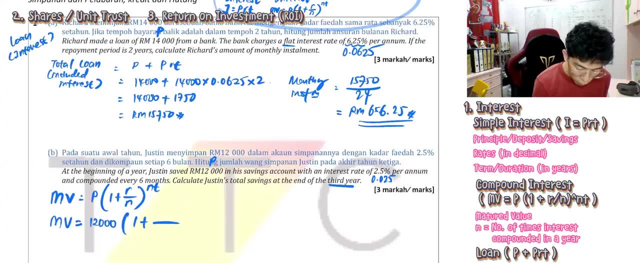 12,000, you know lah, One plus the rate is well, it will be 0.025.. And now, what you're going to put for these few things there, Everyone, let me ask nicely, What is N? 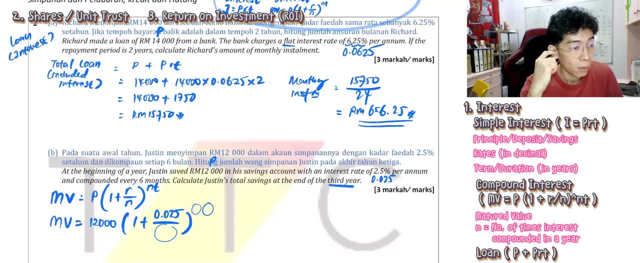 Can you try answering it? Ah, then Jingxuan, because they put the word compounded. mah So sure, compound already. Hmm, Ah, the, the word is like very obvious. then They will say then: Ah, Jinwei, suppose it's correct. 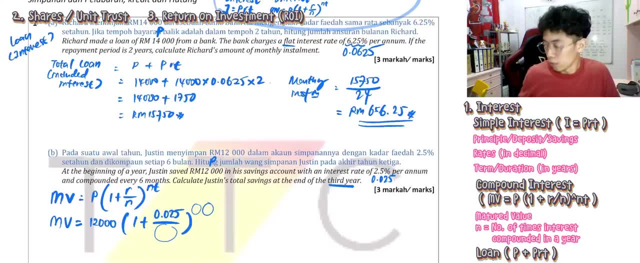 You just have to add the word compounded. Yes, Jing, correct, Ina, specific a bit, Nah, specific a bit, I tell you. ah, Everyone. the question says compounded every six months. Okay, Tell me, in one year the bank compounded how many times? 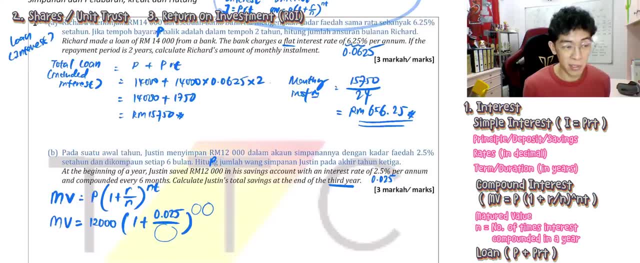 Alicia, yes, yes. And you add one more word: in a year, Ah. then you answer is correct. Very good. So I repeat: ah. N the N formula there. But perfect, Alicia, Okay. So the N over there means ah, compounded how many times in a year? 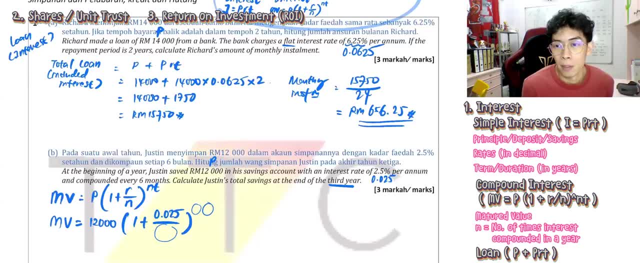 Number of times being compounded. Very good, So every six months. it will be two times in a year lah. So ask you a few more questions. y'all tell me, uh, if i say compounded every month, every month, yeah, 12 compounded every four months. 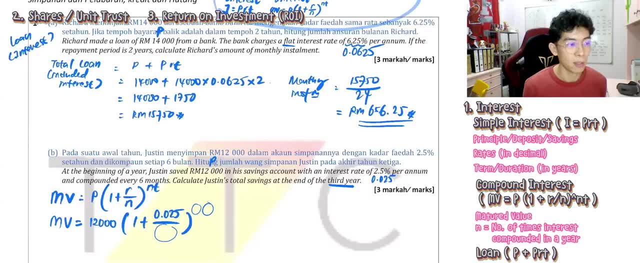 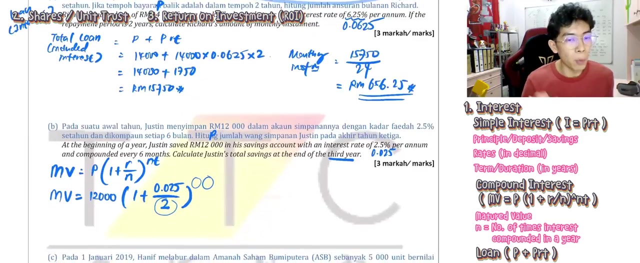 three, very good, compounded by monthly. by monthly means every two, every two to uh, two months. by monthly, it will be six, okay, it will be six, okay. so in this case, your answer will be two and everyone. fair. do you know why they divide by two or not? of course, one of it is because of the given, given info compounded. 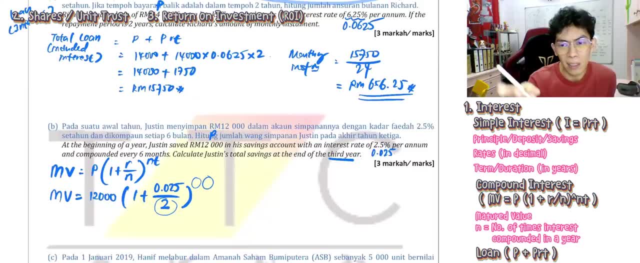 every six months. now why is it to be fair? the reason being a: the 2.5 per annum is for one month, so if you divide by two months you will get six. okay, so in this case, your answer you, you compound every six months. so after six months you have to start compounding it. 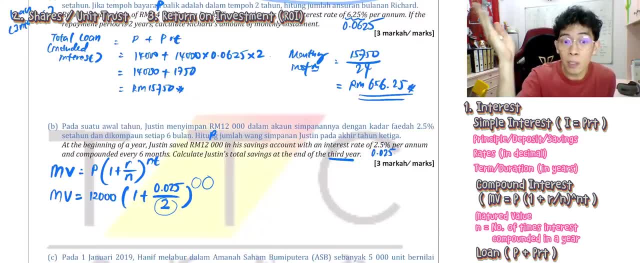 but your 2.5 percent is for one year, you know. that's why they develop by two, fair, so they make it half of it. if i say, compound every three months, you develop by four. so it means you take the 2.5 by four times, then it becomes three months, right? so you're going to. 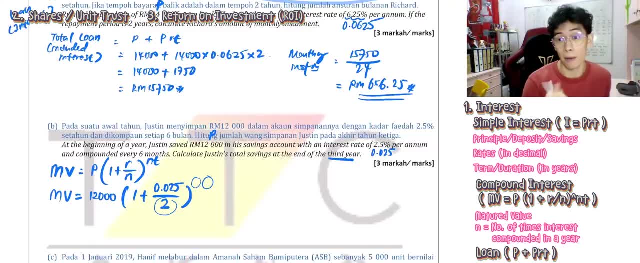 make it half months, right. that's why you develop by two, that's the reason why they divide. uh then, uh, then. the power over here is about n, which is two times with three years, and this is being six. what is the six indicating? the six indicating the total compounded amount throughout the whole. 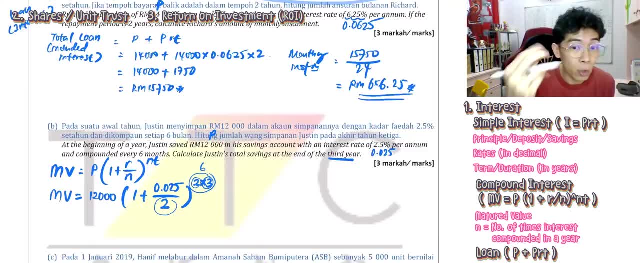 investment. ah, can you see, every year you come out two times and you invest for three, three months, three years. sorry so, two times three, six times, you compounds then. that's why the power six is is to act as a quick calculation of the total amount, of the total amount, of the total amount. 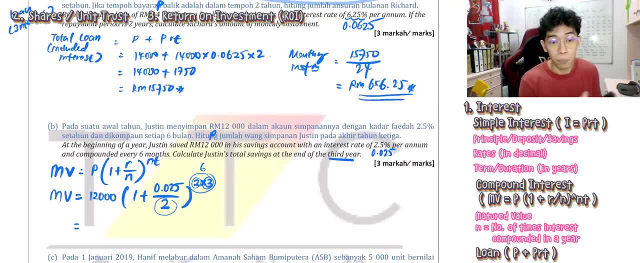 for you. then you hunt them into your calculator. what's your answer? i will recommend student to do this first: calculate this first, and then plus one, and then power six, then only your times with twelve thousand. come, go ahead and tell me the final answer. twelve thousand nine hundred twenty eight point six zero. point six zero. that's the answer. 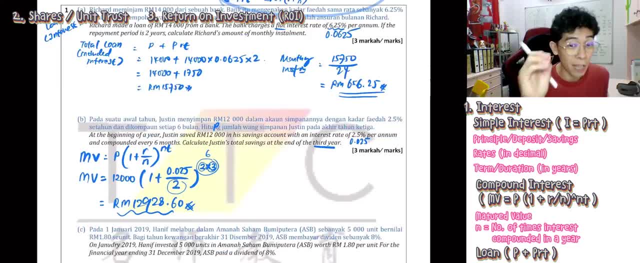 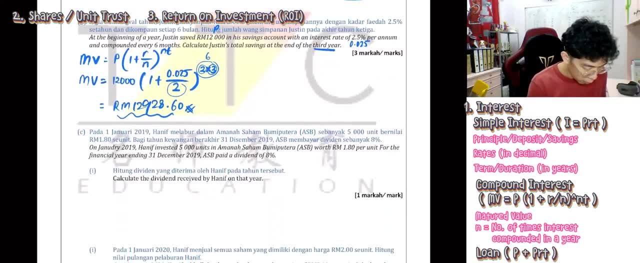 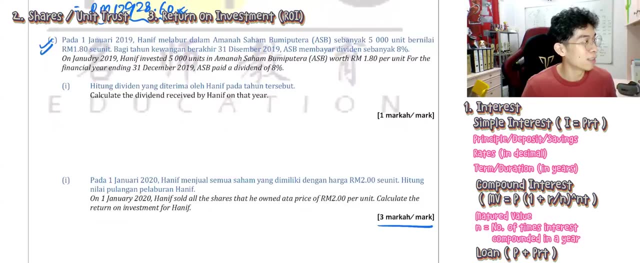 so we do one relating to shares and it's about roi as well. okay now, so we do another one in question c. all right, question c on janet jenner dry, generally dry, on janet dry. okay, what happened what it says? okay, it says: uh, panif invested five thousand units in amana, in amana, what amana saham? 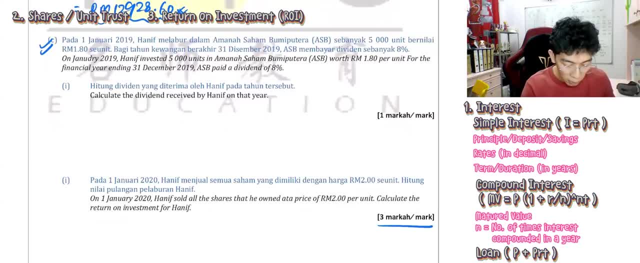 bumi putra asb worth 1.8 unit. for the financial year ending 31 uh 31st december 2019, asb paid a dividend of eight percent. this one's simple and can you see? one, one, one mark only. so i just quick one, uh five thousand times. 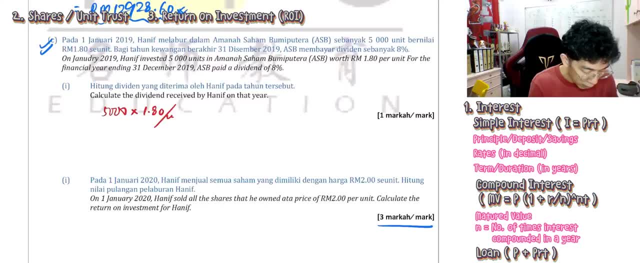 with per unit: 1.8. okay, 1.8. this one is rm. uh, this one is five thousand units and you will get rm nine thousand. so the rm nine thousand eventually, you have to times with because the dividend paid out rate is eight percent. uh, so times with zero point zero eight. so what is the dividend count? 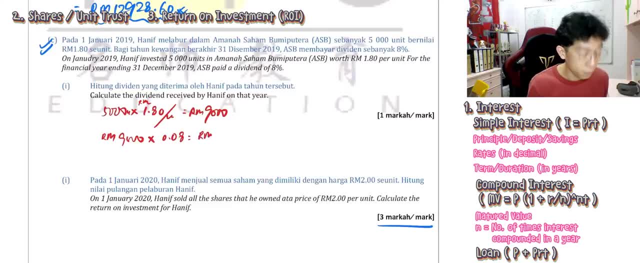 come on y'all, let me just check for one second. seven hundred and twenty, that's the dividend. wait, wait, everyone is 720 the dividend. a return to hanif. is that a return? yes, it's a return of something that you receive. you invest something you want to return you. 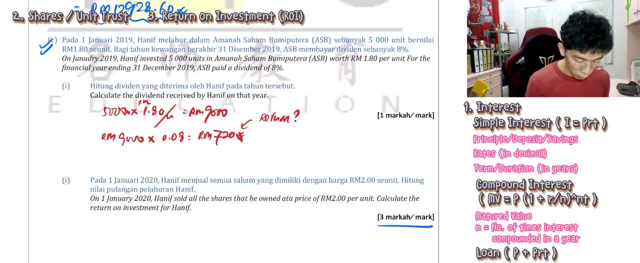 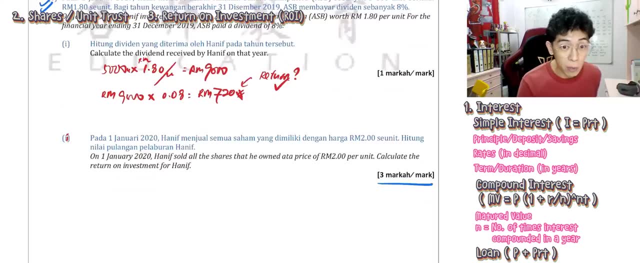 invest something, you get lost, then what? no point mark to ignore? ah, so that's a return, yes, okay, now the the second one. sorry, this one second. uh, on first january 2020- it means the next year, exactly one year- hanif sold all the share. hanif sold all the shares that he owns at 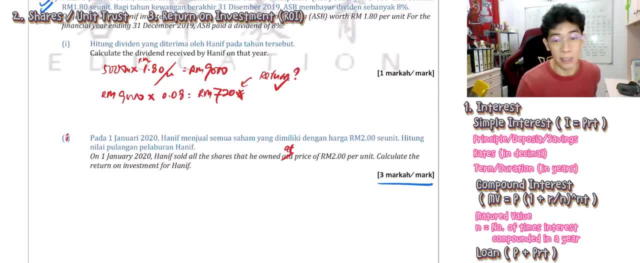 at price, at a price at a price of two ringgit per unit a. did hanif earn something originally, buy at one ringgit, 80 cents, right, and sell it for two ringgit, or so can you tell me. per unit of profit is how much? per unit of profit is 20 cents, correct? so that's a. that's a returner. so the total return? 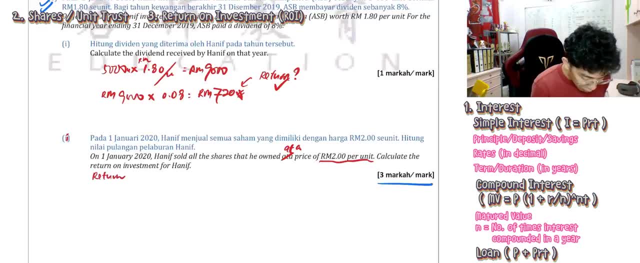 sorry, i say return better. the return equals to rm rm 0.20, rm 0.20, rm 0.20 times with 5 000 units, the return is rm 1000, 1000 return by selling all the given share. because they say sold all the shares already. mark right now: hanif sold all the shares. 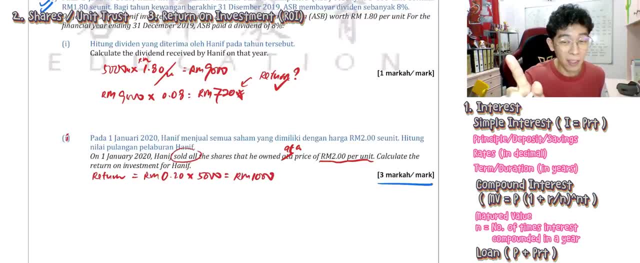 calculate the roi. tell me what is the total return. i put the formula over here: total return divided by initial investment times: 100. what is the total return? besides the 1000 as the return, what else? the 720 dividend: it's also a return because one and two link on, so you have to add the 720. this. 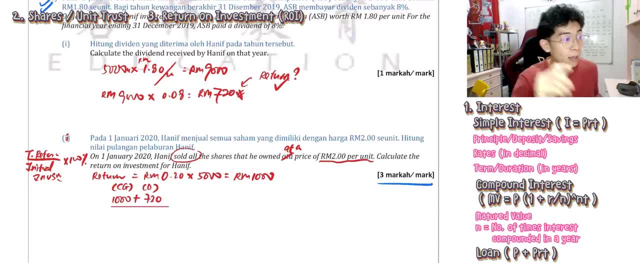 is the dividend. this is the capital dividend. this is the capital dividend. this is the capital dividend. it's not part of the stipend. but you lose, because if you win, you lose your capital gain. so you really need more capital gain here in second half of ah. so 1720 divided by 9000, and then times 100 percent, wow, 19.11 percent. so everyone can you. 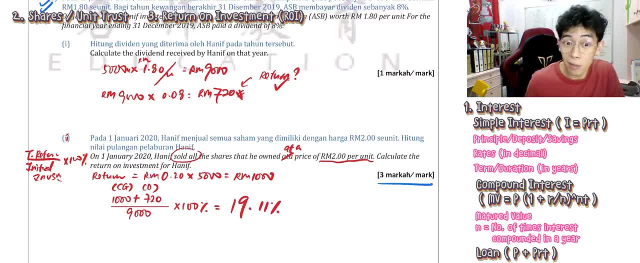 see the, the, the, the share investment is 19.11. okay, ma worth it. it's still better than fd, right, but fd is like kind of fixed already and it's like confirmed. you get that that percentage. but for shares, right, there is a risk there. so you have to analyze, you have to really study then. 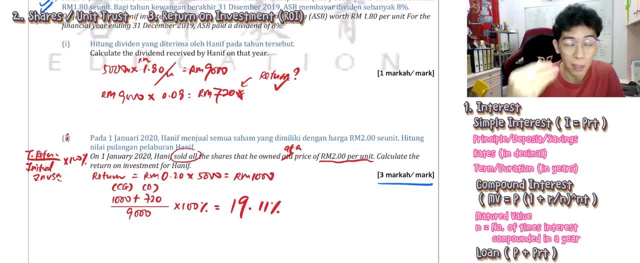 only you can gain the very high return, uh, in the percentage. okay, so that's about risk. is your form three? um, objective related informations, that will be two in that ready. so everyone, i'm gonna stop here today. um, i believe today class you'll gain something. okay, if you're not so sure about it, you.